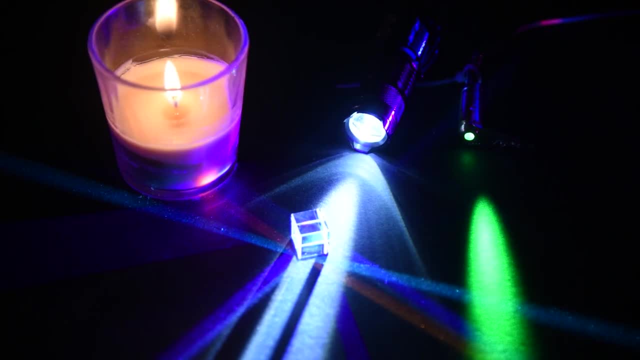 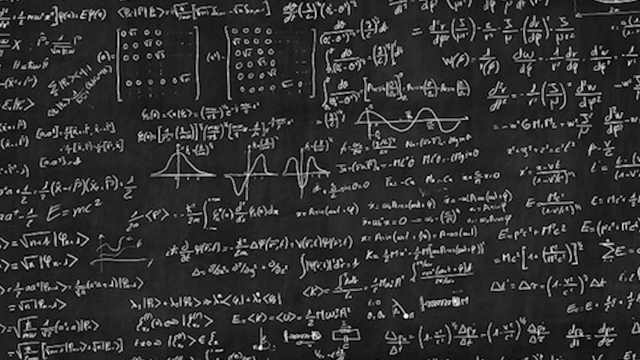 the moon. Got all that Good Moving on, Let's start simple. What is light? This is the part where the physicists collectively panic because that answer is surprisingly complex, but we're going to stick with the basics. Light is composed of particles called photons. The bit where 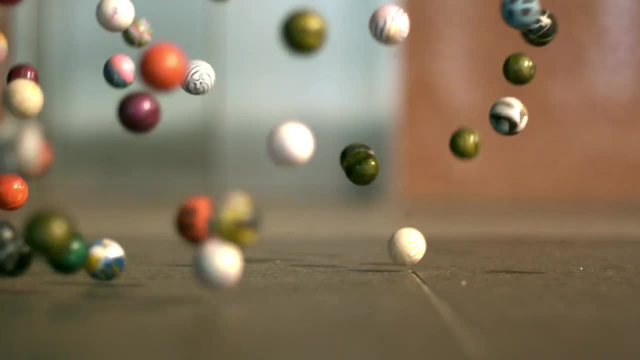 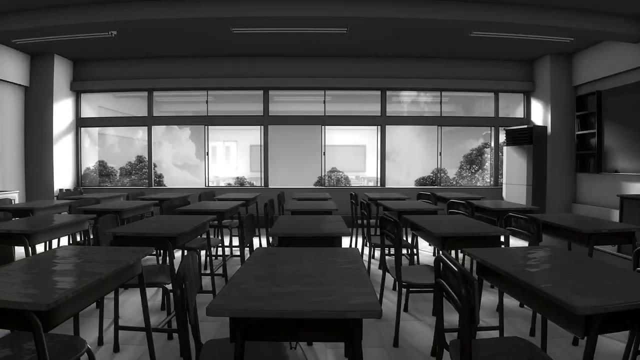 it gets weird and the physicists start sweating- is that, even though photons are particles, they behave like waves. That probably sounds convoluted, so let's do a quick experiment to see what this looks like. If you've spent any time in a physics class, you've almost 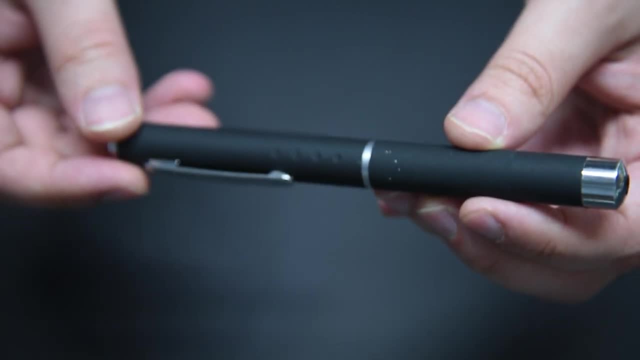 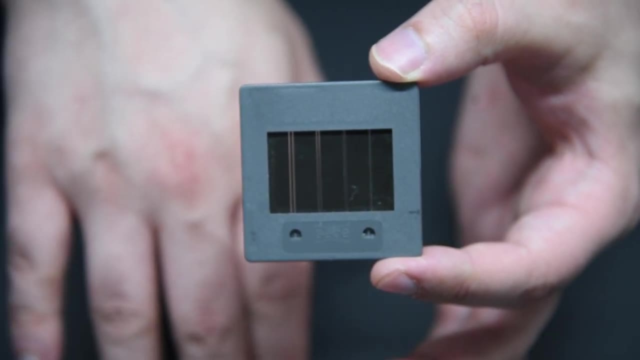 definitely heard of the double slit experiment. The idea is pretty simple. You've got a light source- in this case I'll be using this little red laser pointer- and a slide with a pair of very fine slits cut into it. We shine the laser through the slits and project the result. 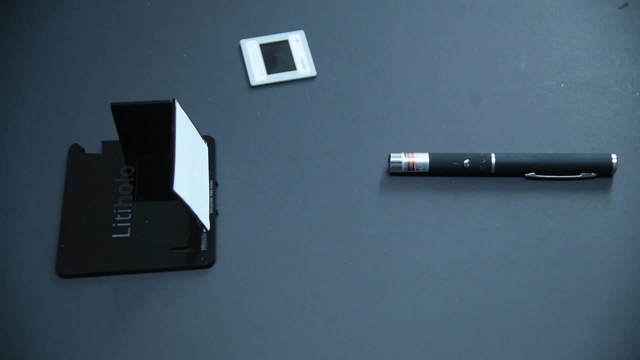 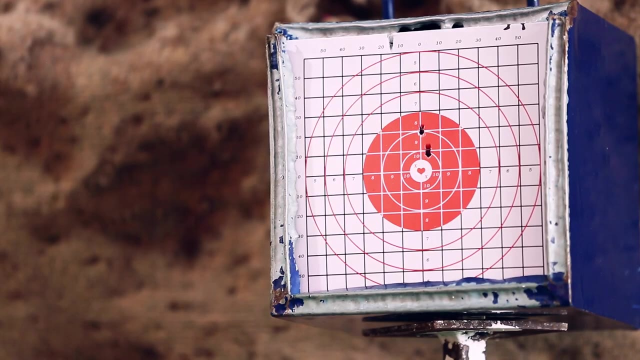 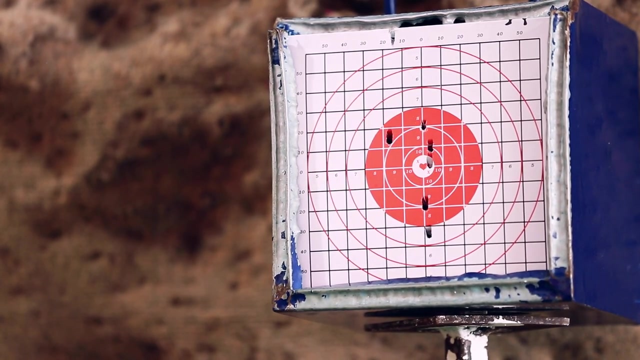 onto a board and, depending on what it does, we'd know if photons behave like particles or like waves. Think of this like the difference between shooting a BB gun and ripples on a pond. BBs would follow straight lines and if they bump into something they stop, But ripples can. 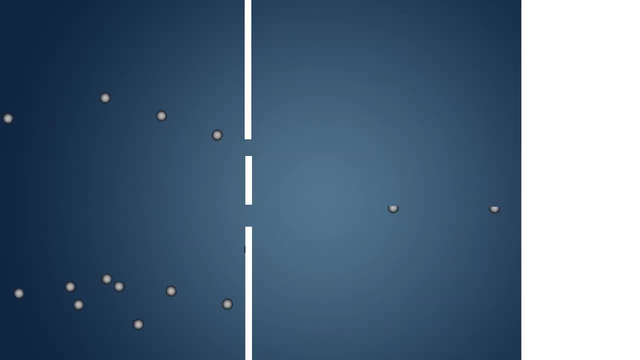 bounce off of things, make new ripples and go around things. In the context of double slits, if you shot enough BBs, you would end up with two lines of impacts on the screen, Whereas with the ripples right after the slits, two new sets of waves form And where. 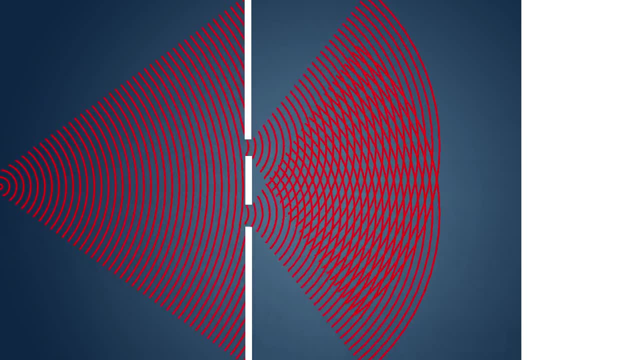 parts of those waves overlap. they'll either add together or subtract, depending on if it's the peaks or troughs of the wave. If you shot enough BBs, you would end up with two lines of impacts on the screen, Whereas with the ripples right after the slits two. 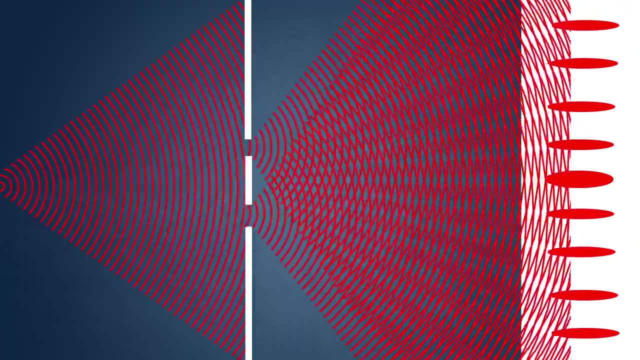 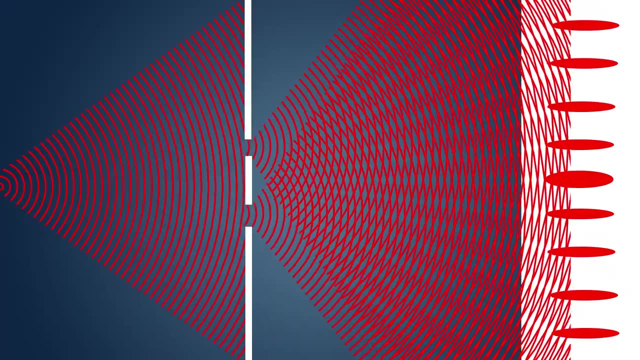 lines of the waves form. they'll separate out of the waves that are lining up. When the ripples hit the screen, certain areas would be struck by combined peaks and others by troughs. In the context of light, troughs would look darker and peaks would look brighter. 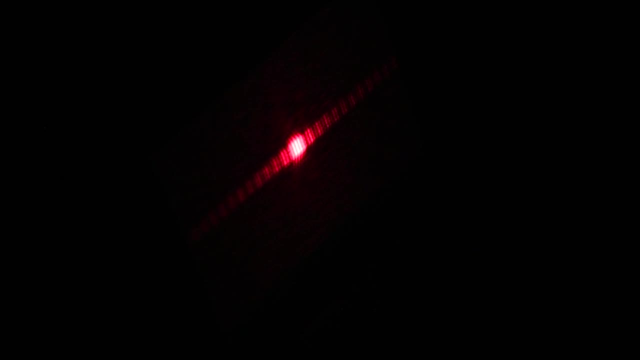 So when we actually do the experiment, what do we get? Well, we get many lines and a pattern known as an interference pattern, meaning light is wave-like. The reason I say photons are particles is because we'd actually get the same result if we fired one photon at. 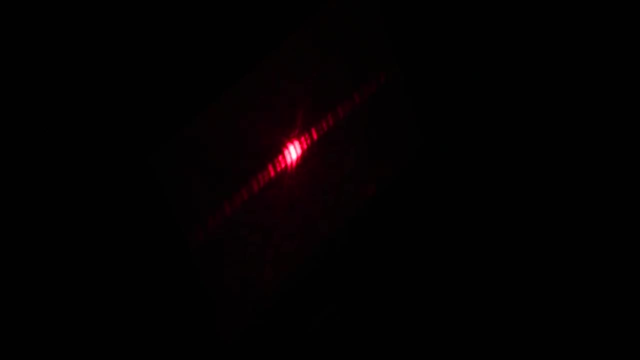 a time, Each individual photon would hit a specific spot in the screen, but as you fired, eventually the net result would be that same interference pattern. This is what I meant by things get complicated. I think the best way to think about this is sort of like waves of water. Even though water is made of individual molecules, you can still make waves with it. It's definitely not a perfect analogy- light is way weirder than that- but I think it helps visualize it, Because light has wave-like properties. that means it also has a wavelength. 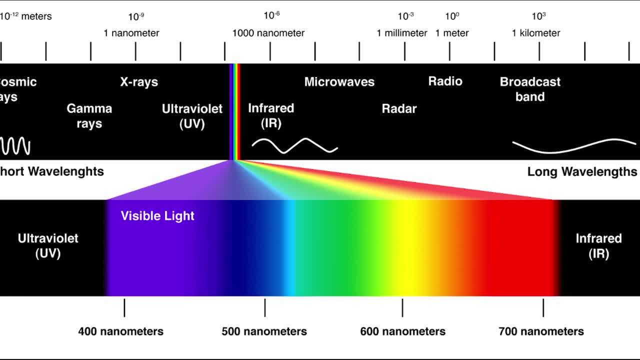 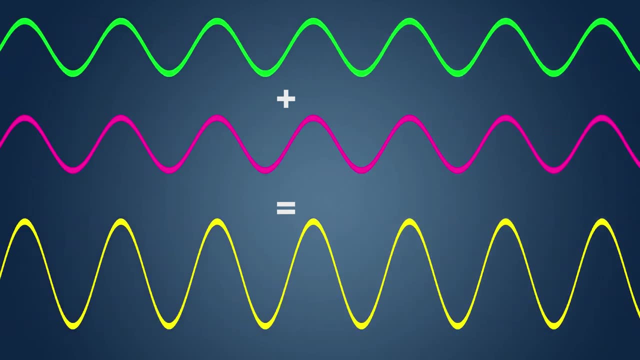 And for visible light. this is measured in nanometers. To our eyes, different wavelengths of light look different colors. Longer wavelengths look red, while shorter wavelengths look more blue. Now, one of the many properties of waves is something called phase. Basically, when you've got two identical waves, if the peaks and troughs line up perfectly, 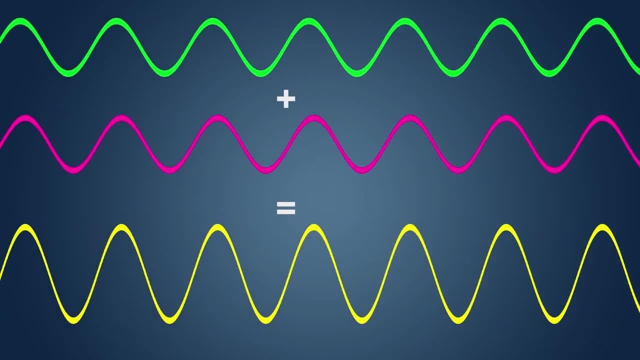 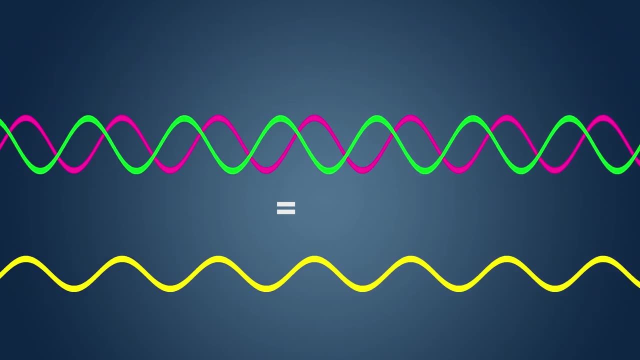 they're said to be in phase and will simply add together perfectly. But if they don't quite line up, they're what's called out-of-phase and different parts will add or subtract less evenly. We measure the phase difference in degrees. This is just an example. 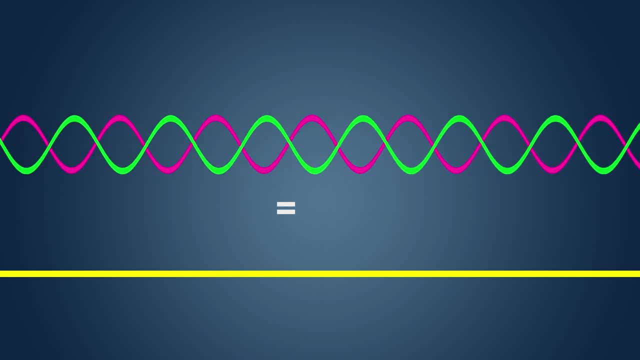 This is just how shifted one is relative to the other. Looking at the simple example of two identical sine waves, if you shift one of them so that the peaks perfectly line up with the troughs of the other, they're said to be 180 degrees out of phase and would actually completely cancel out. 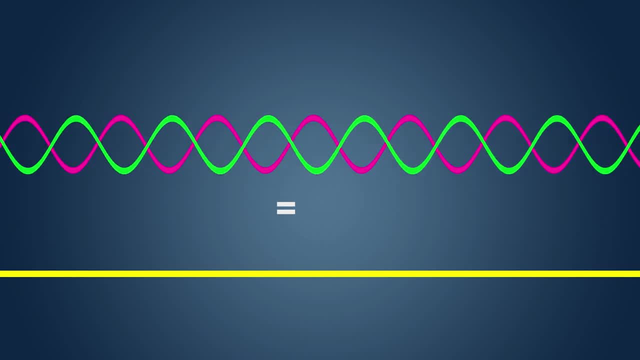 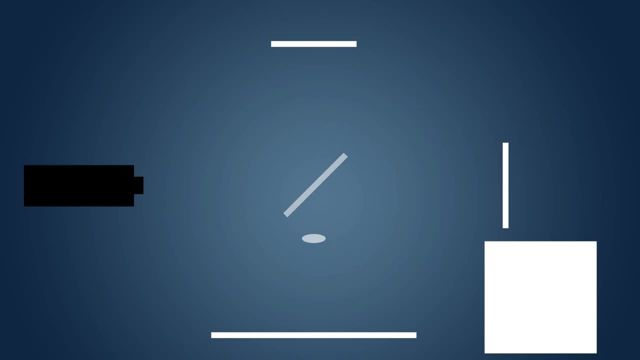 The same thing applies to non-identical waves, but this simplistic case makes it easier to understand. Now let's see how this works in the real world and do another experiment to see how phase can affect light- And don't worry, this is the last one- and then we can make some holograms. 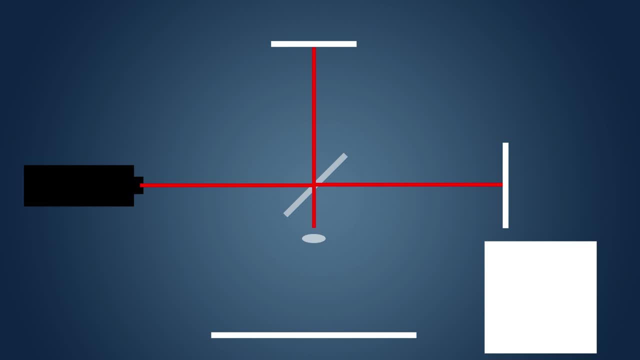 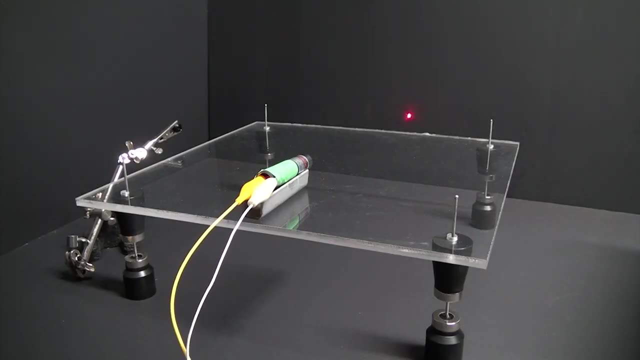 We're going to be setting up what's called a Michelson interferometer. It's quite simple but has a few more pieces than the double slit experiment. Again, we're going to be using a little laser pointer as our light source, and we'll talk about why that's important in a moment. 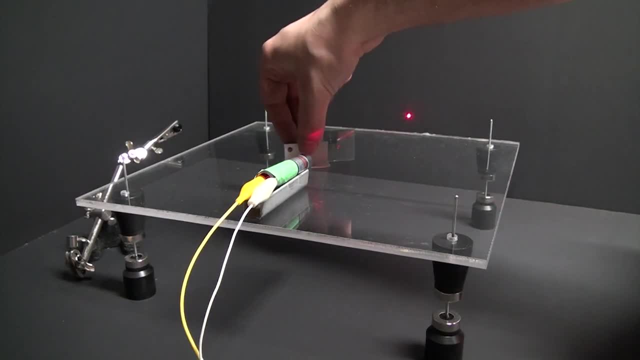 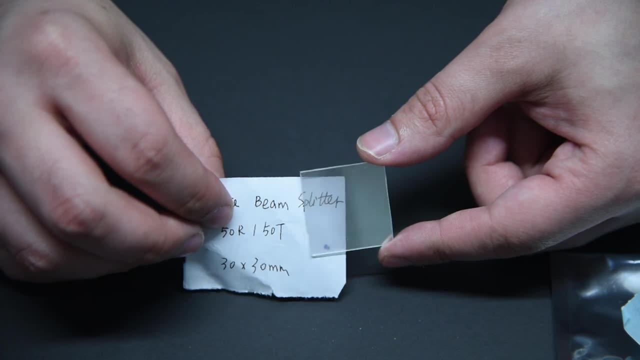 Then we've got what's called a beam splitter. Basically, this is just a mirror, but when they applied the silver coating to it, they only made the metal layer thick enough that about 50% of the light is actually reflected. The rest goes right through as if it was an ordinary piece of glass. 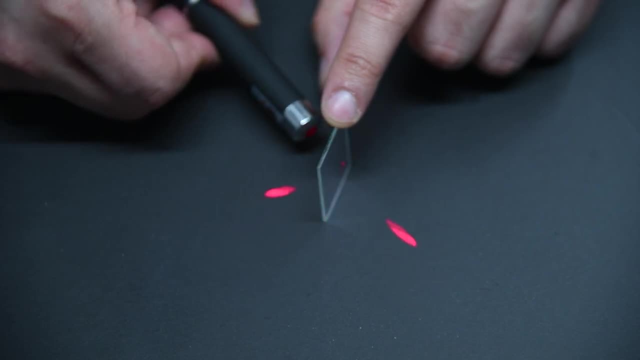 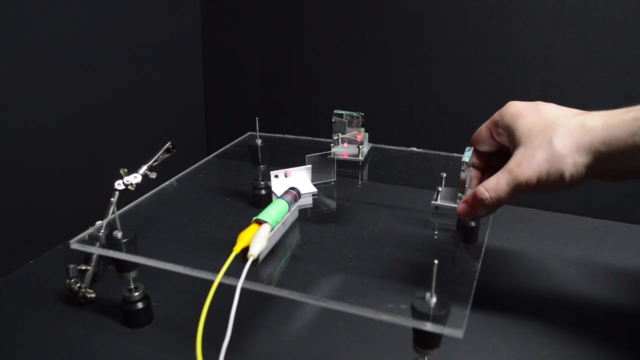 This takes our single input laser beam and splits it into two new beams. These two new beams are then each bounced off of a mirror back to the beam splitter, and it's very important that the two mirrors are exactly the same distance from the beam splitter. 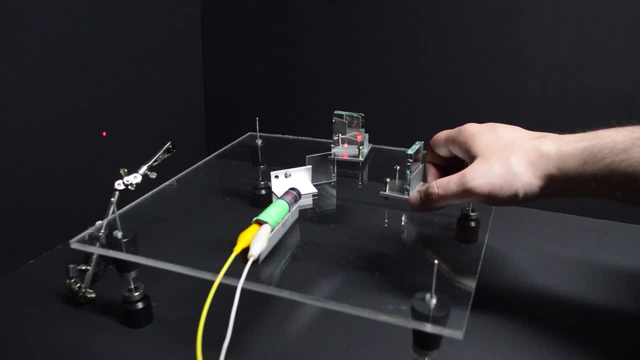 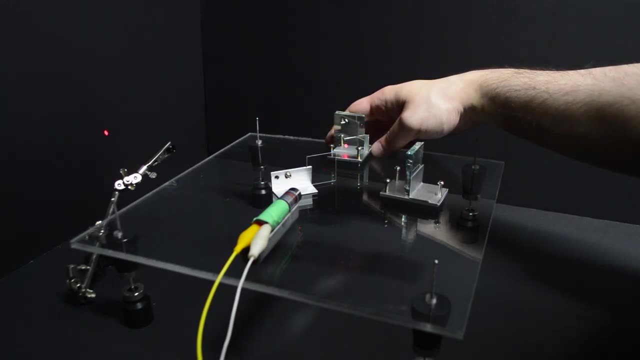 Again, this splits each beam in two. Two of them will be heading vaguely towards the laser pointer and two will be heading towards the screen which we'll be using as an output. If we line everything up just right, these four output beams can actually be combined. 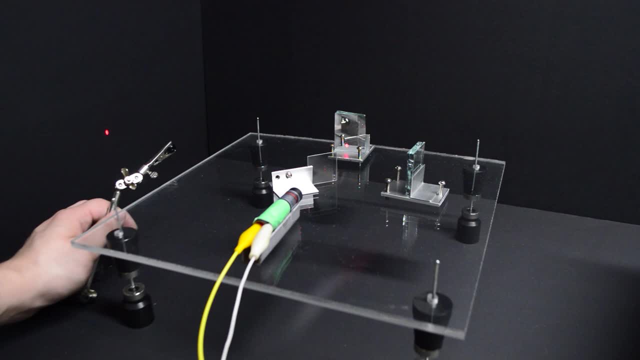 simply into two overlapping ones. One is heading towards the screen and one towards the laser. We can ignore the one that's heading towards the laser. It's hard to see the result of what happens when the laser beam is tightly focused on the screen. 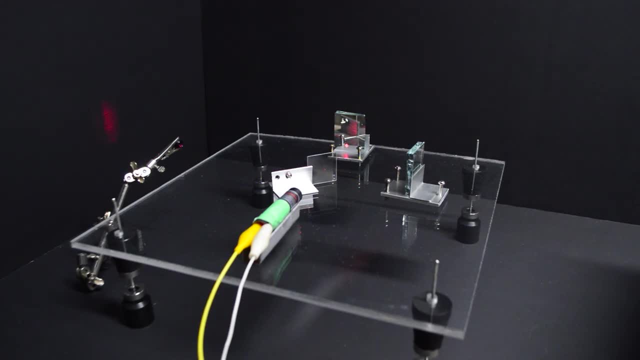 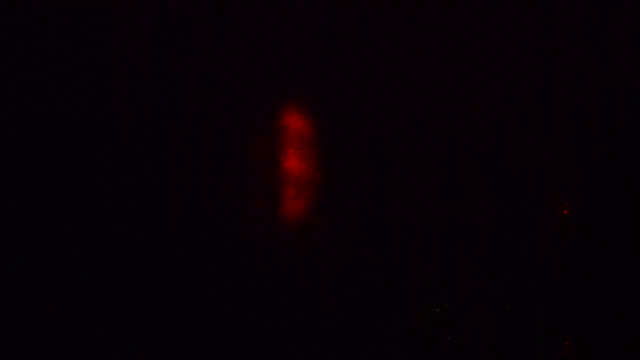 so a simple magnifier lens is used to expand the beam, so we can see what's going on, And what we see is an interference pattern like before. So what's happening here? Well, laser light has two properties that make this possible. 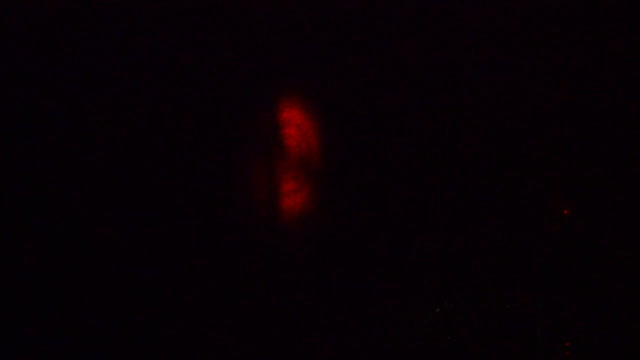 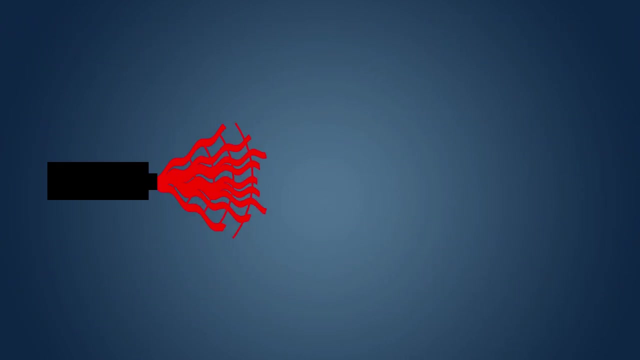 First, most of the light from the laser is the same color, ie the same wavelength. This makes it resemble that idealized example before of identical sine waves. And second, the light is what's called coherent, which means that when the photons leave the laser, 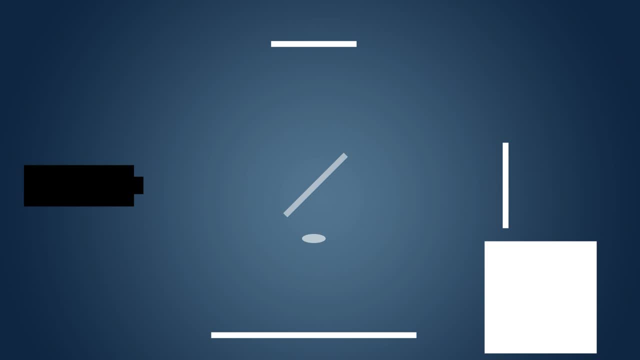 they all start off in phase with each other. When the beam hit the beam splitter, the two sets of photons each had to travel to a mirror and back before being recombined on the output. But my setup is far from perfect, so each beam had to travel a different distance relative to the other. 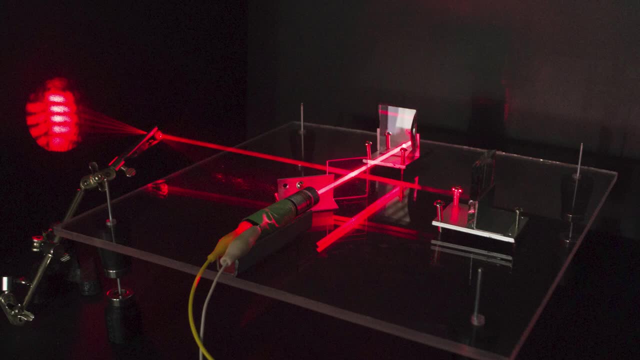 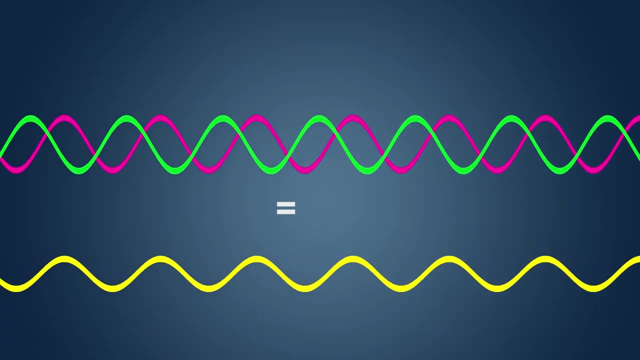 And the alignment of the beams isn't perfect either, so they don't perfectly overlap. As such, one of them is slightly delayed and offset relative to the other, so the phase of the two beams is now slightly mismatched. And when the phase is mismatched, 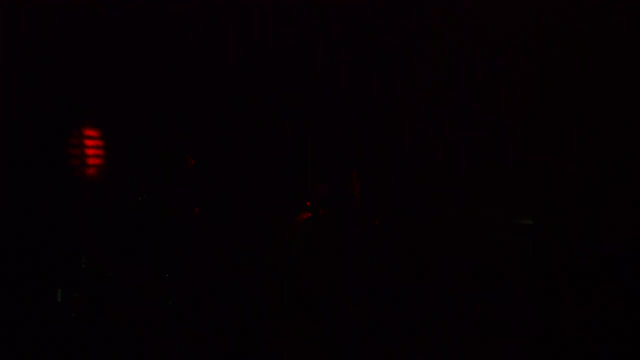 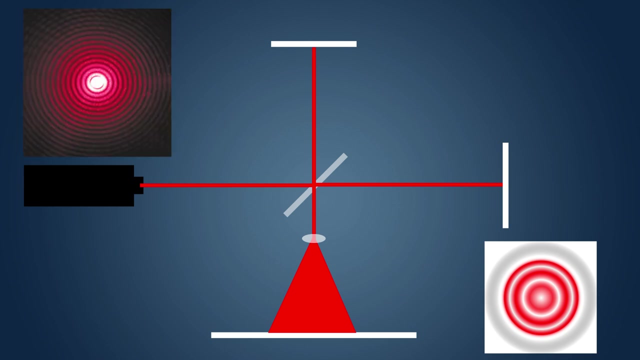 the waves don't add together perfectly, So some areas look dark while others look lighter. In a professional grade setup, where the alignment is much better, you would actually see rings, And the number of rings corresponds directly to the difference in path length between those two mirrors. 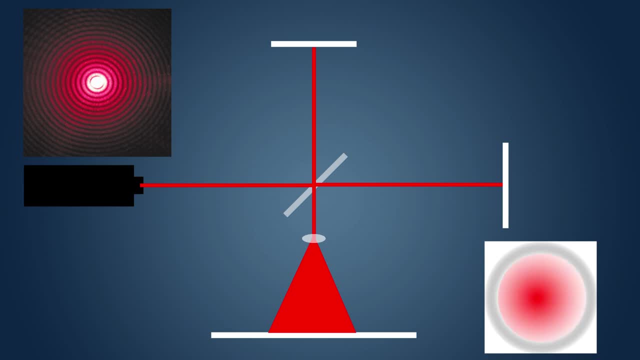 If you get everything absolutely perfect, the output would either look like one solid bright spot or complete darkness, which does look very odd when you can clearly see the laser beam hitting that spot. But I'm doing this with cobbled together garbage, so you can just see sets of lines. 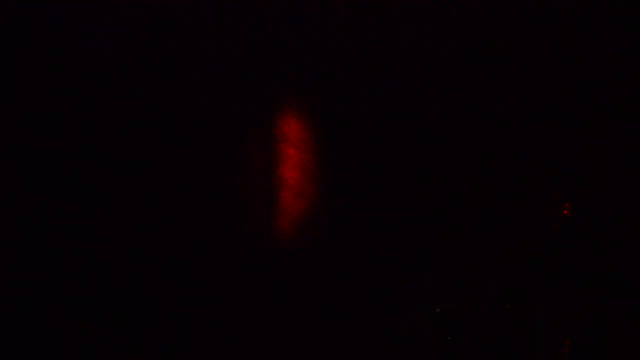 Also. one last note is that the pattern is extremely sensitive to vibration, because any motion moves the mirrors and thus changes the pattern. This will be important in a moment. Okay, finally, we can look at holograms. There's actually a few different kinds of hologram. 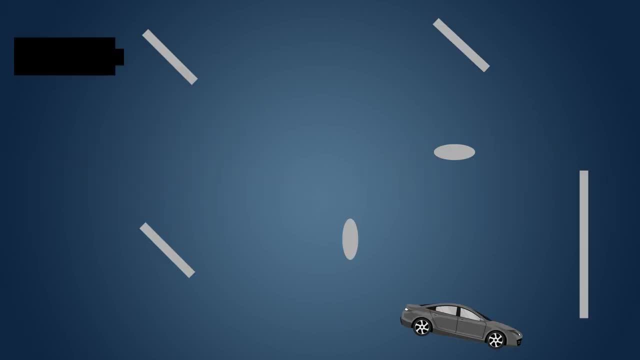 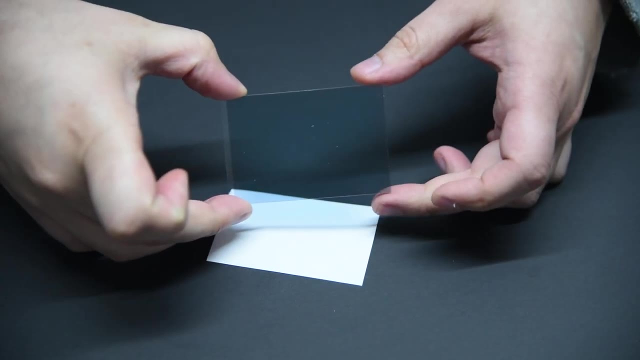 but they all work on basically the same principle. The basic idea is very similar to the interferometer, but with a few key changes. First, instead of a screen, we're going to be using a special type of film that can capture the interference pattern that forms. 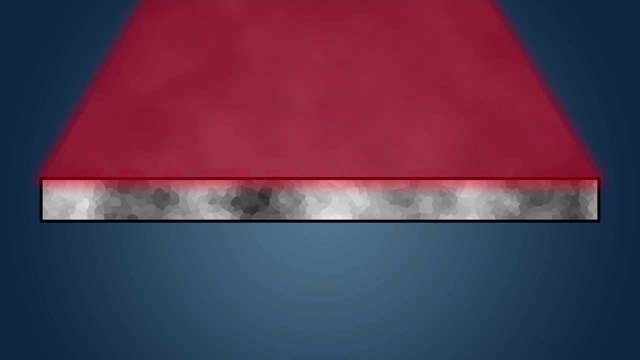 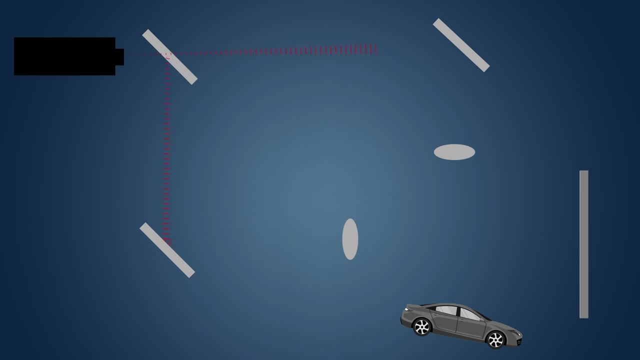 so that we can look at it later. We'll talk about how that film actually records the pattern in a bit. Again, we split one starting beam in two, but instead of bouncing the two beams off of two identical mirrors, one beam is sent directly to the film. 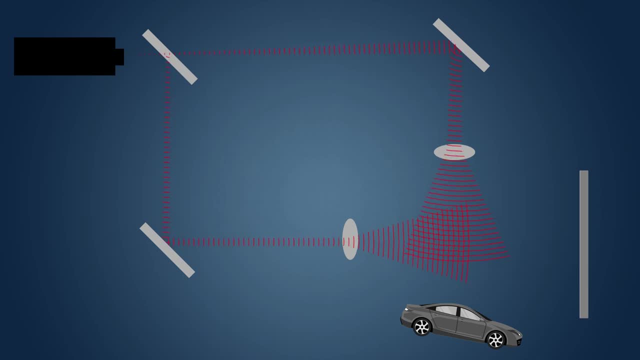 usually by bouncing it off a mirror, while the other is reflected off of an object instead. Also, instead of only expanding the beam at the very end, in this case, we expand each beam so that, once it's been reflected off the object or mirror, 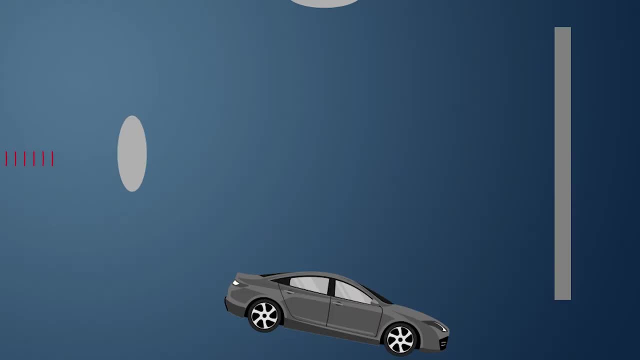 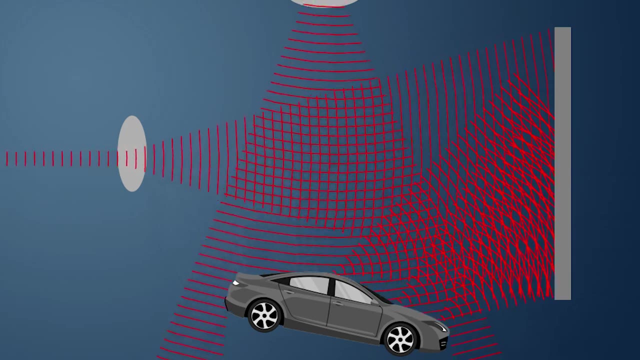 it covers the whole area of the film. Just like how small differences in the mirror position change the phase of the light. each point on the object is going to be a different distance from the film, So each point on the object will change the phase of the light that hits it. 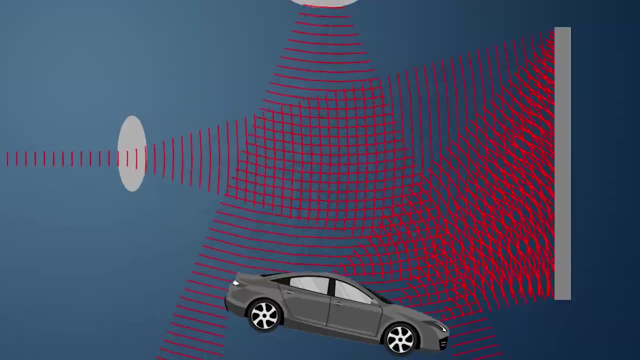 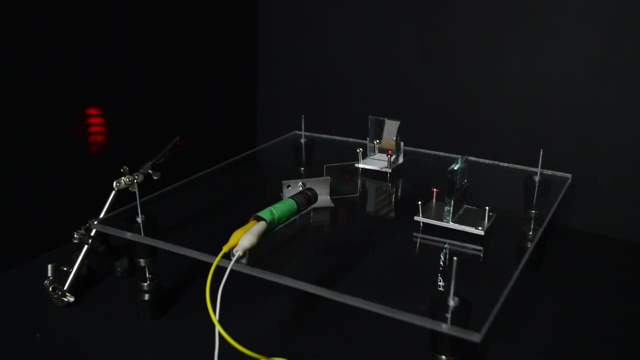 And when it strikes the film it'll interfere with the other beam and create a pattern. We call the beam that bounces off the mirror the reference beam and the beam that bounces off the object the object beam If we think back to the interferometer. 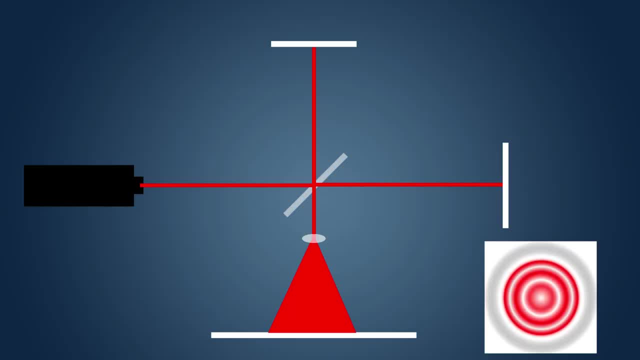 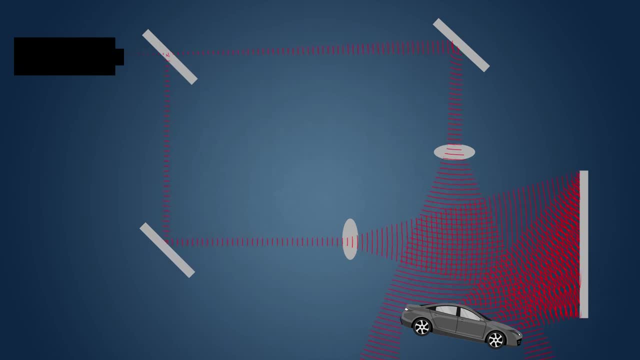 usually the professional version where you get rings. the pattern is simple because only one dimension is really being measured: the difference in distance of the two mirrors. But with a hologram we're measuring three dimensions, so the pattern is much, much more complicated. 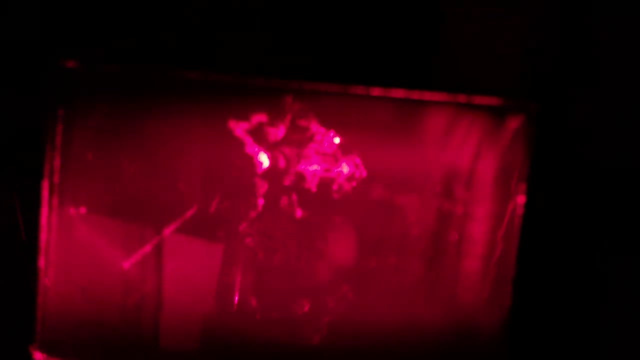 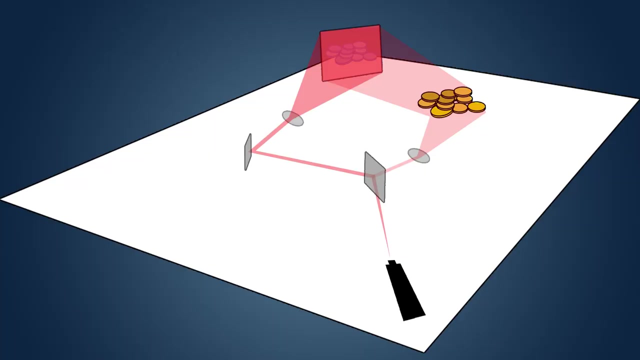 But the end result is that all of that 3D information of the object gets encoded in that pattern. So when we view the film on its own, we can see the object as if it was in front of us. Now the method I just described of splitting a laser into two beams- 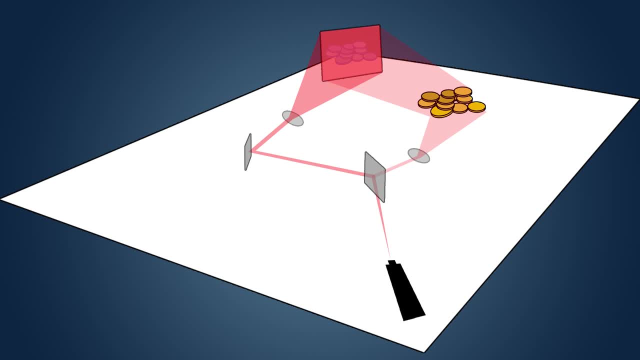 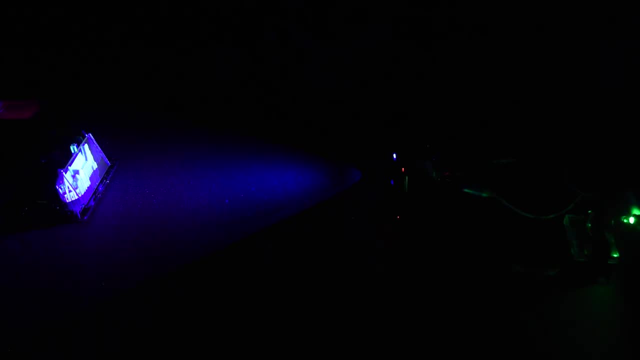 and using a mirror and lenses is fine and well, but it's quite challenging to actually do without a very expensive setup and is quite fiddly to get right. But, like a good scientist, I prefer methods which are easy and cheap whenever possible. 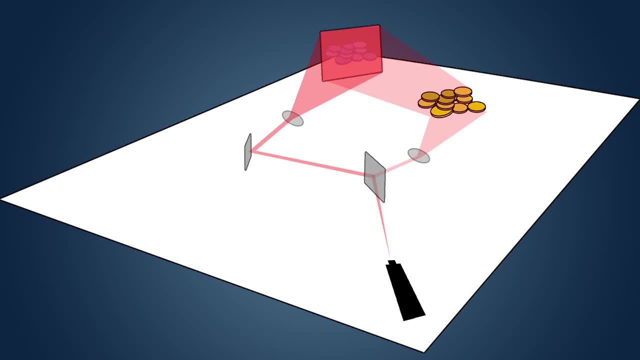 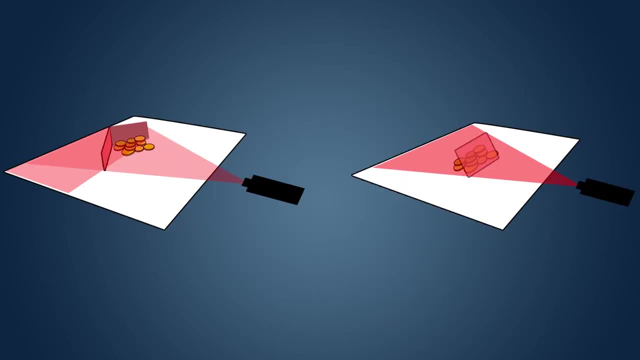 and thankfully such a method exists. The theoretical version I described is what's called a two beam hologram for fairly obvious reasons, But what we'll be doing is called single beam holograms. Basically, we're sort of cheating and making one beam act like two. 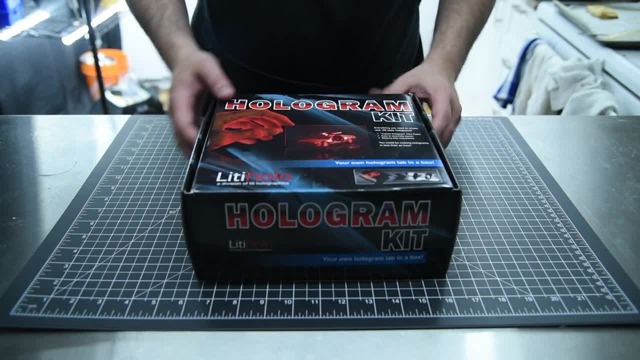 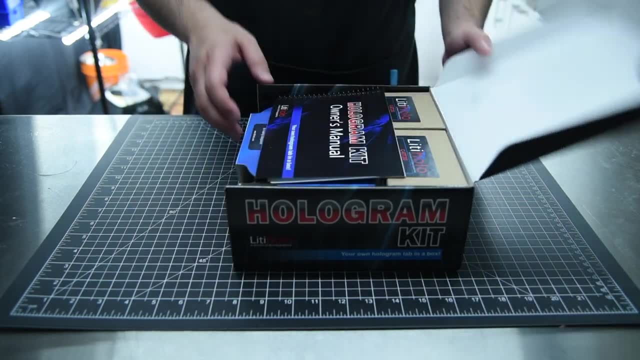 by setting things up in just the right way. Before I go further, I actually need to take a moment to talk about an amazing company called Litty Holo, which was kind enough to supply many of the materials you're about to see me use. 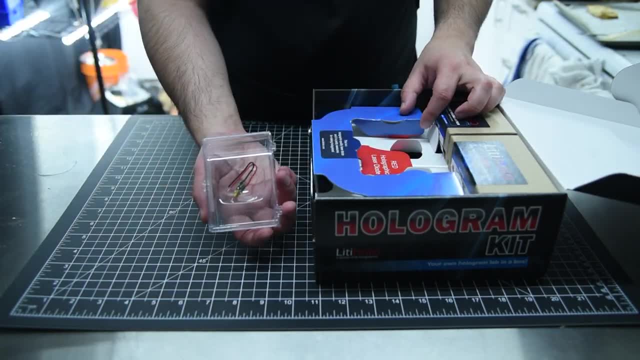 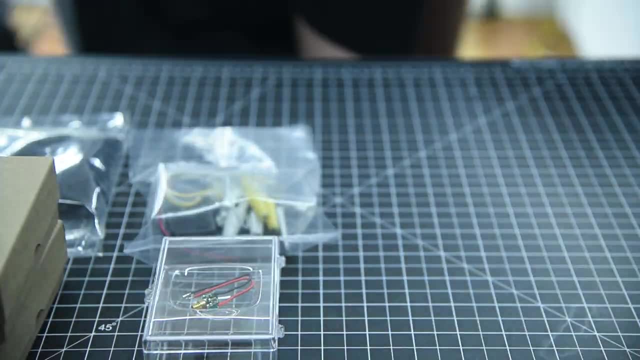 Originally their company made kits for making holograms at home and they were actually kind enough to send me not only their original kit but two of their upgrade kits and a pile of extra hologram film for me to use in this video. And I should say that the film they sell and will continue to sell. 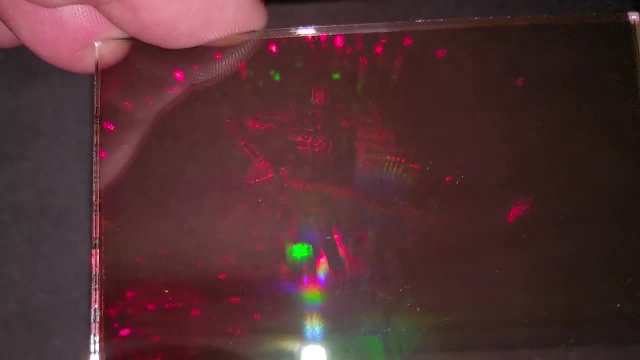 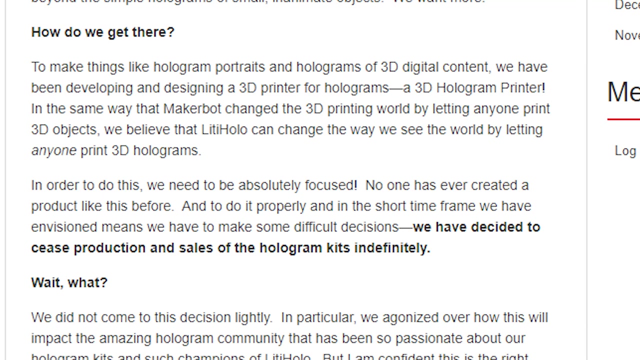 is by far the easiest hologram making material I've come across and is quite cheap. Unfortunately, they're discontinuing their kits, but are actually working on something even more amazing instead, which is a hologram printer, The idea being that you can just give the printer a 3D file you want made into a hologram. 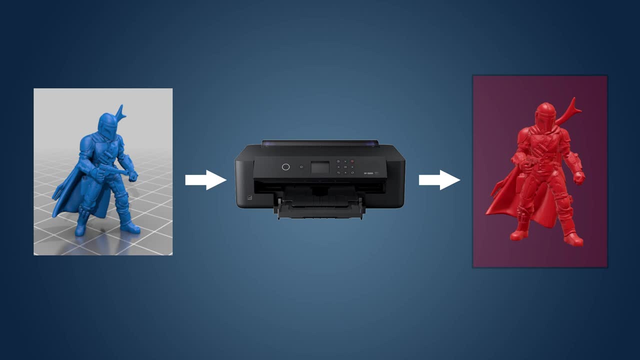 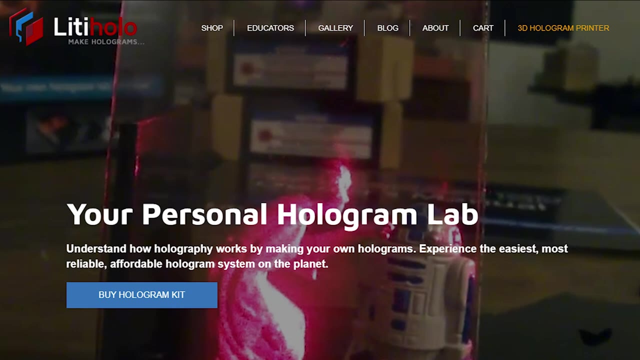 and it'll spit out a hologram just like how a regular printer works. It's really a very cool idea and I hope one day I can show it off on the channel. Links to all of their stuff can be found below, and fear not. 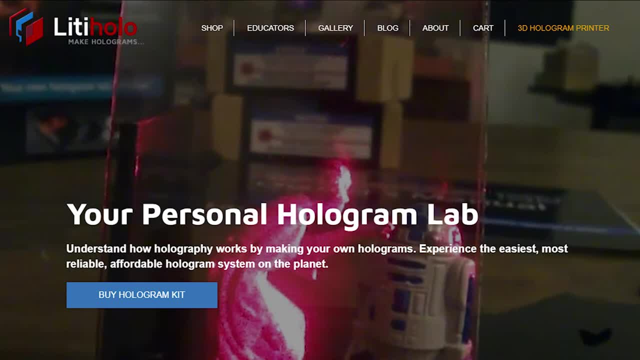 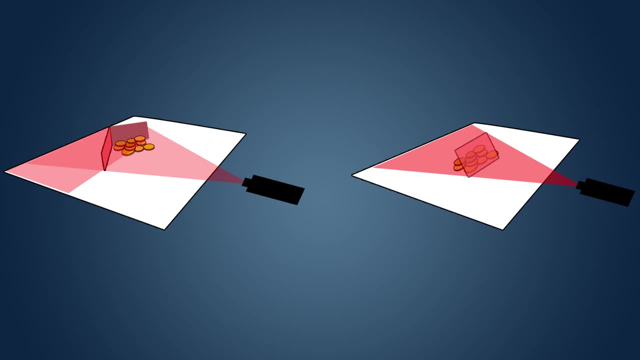 as long as they continue to sell the film, you can make holograms using the method I'll show, even without the kit. Okay, back to making holograms. Like I said, we're going to be making single beam holograms, but we still need to decide on the precise setup we'll be using. 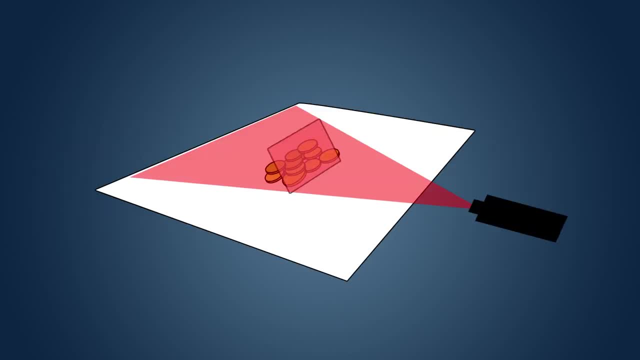 You see, holograms can really be divided into two types: reflection and transmission holograms. and this has to do with where the light source needs to come from in order to see the finished hologram. In a transmission hologram, the image needs to be backlit with laser light. 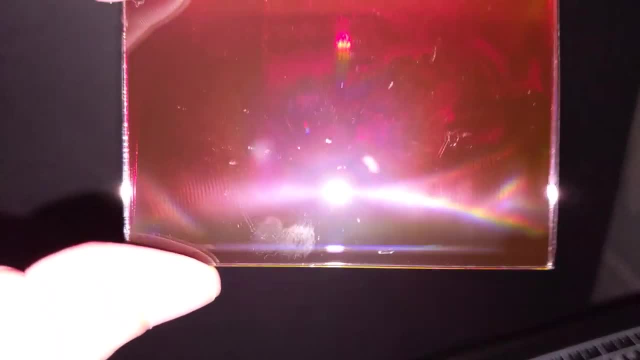 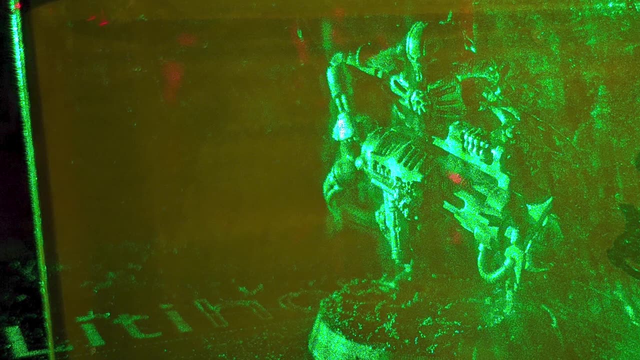 in order to see the final hologram, whereas reflection holograms can be lit and viewed from the front. Personally, I prefer the latter, but we'll be making both types so you can see the difference And once we're used to the fundamentals. 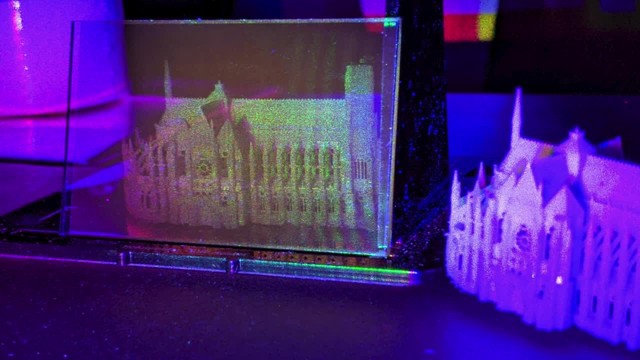 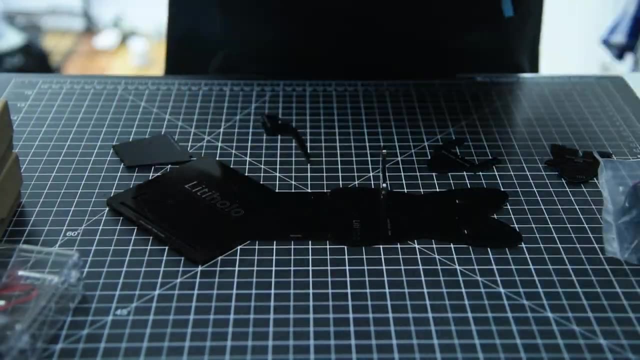 we can look at other colors and the rainbow holograms I showed at the beginning, as well as other recording media and how they all work. But let's start simple. I'm going to be using the original kit, set up exactly as it was intended. 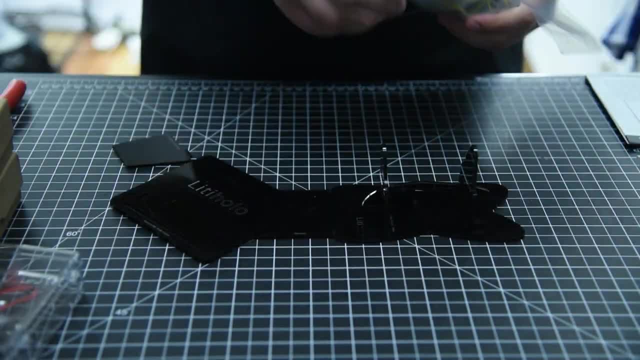 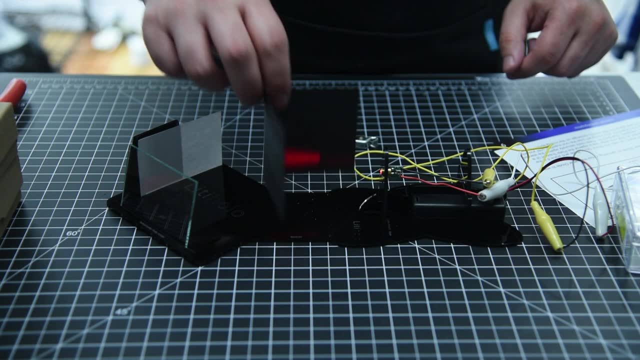 and this means making a transmission hologram. The kit comes with some beautifully laser cut acrylic pieces that just snap together a red laser diode and a battery pack. This diode has no lens on it, so the beam automatically spreads out into a nice vaguely rectangular beam. 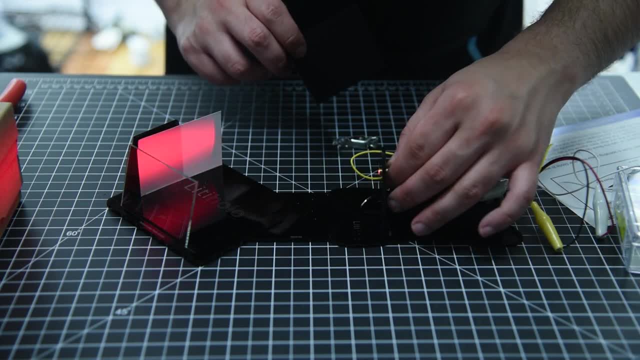 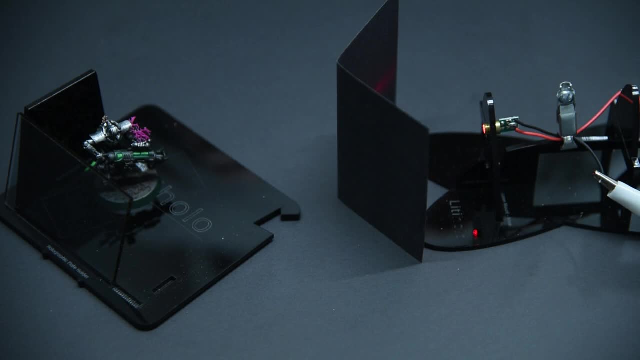 that'll cover both the object and the film plate. The kit is divided into two parts: the laser mount and then the object slash film holder. There's a spot marked on the base plate of the film holder where you can place an object. 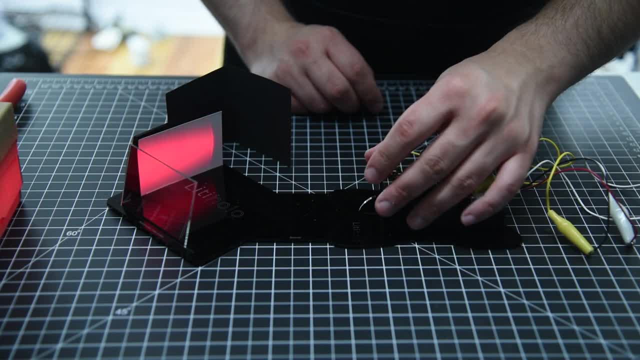 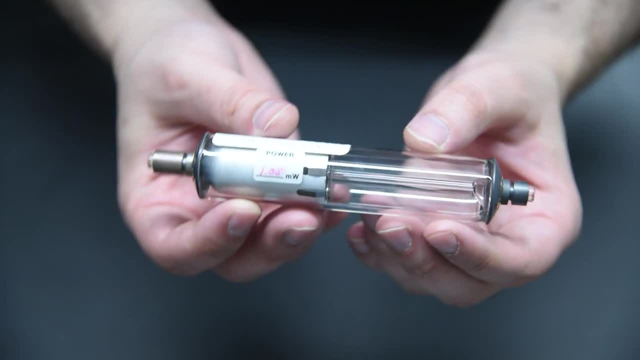 and a slot for the film. When I was first planning this project, before I reached out to Liddy Hollow, I was under the impression that you need super high quality lasers and equipment for doing this. So I picked up an old school helium neon laser tube. 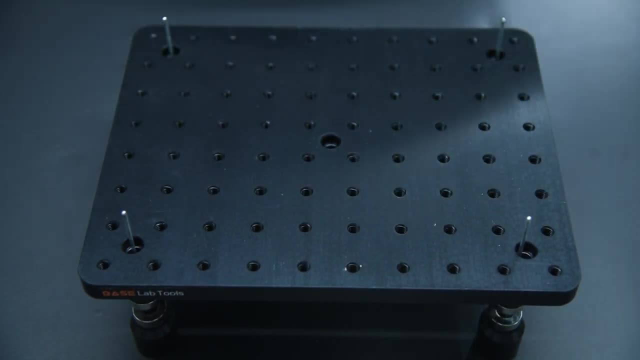 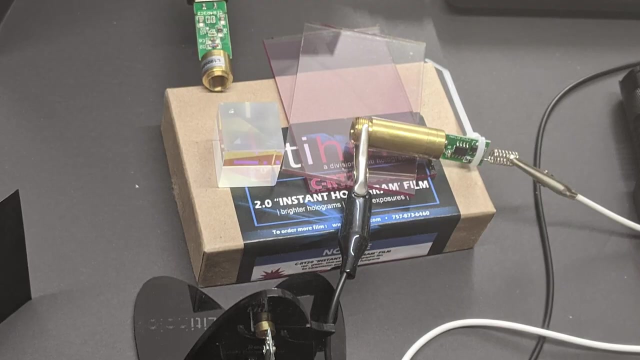 and even made a video about making a magnetically levitated laser table, Which you saw me use for the interferometer. But, as you'll see, none of that is actually required In the end, all the lasers you're going to see me use. 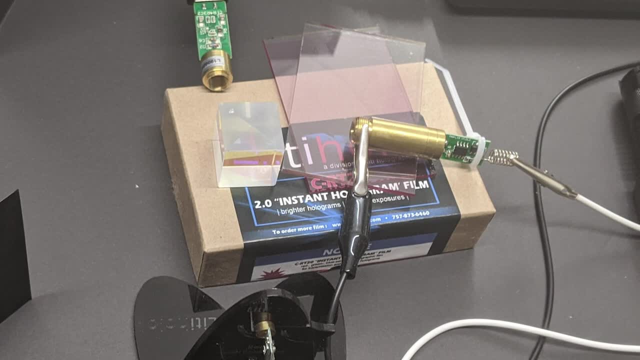 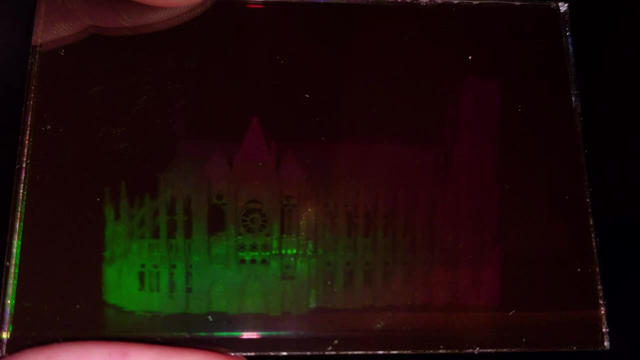 were purchased for a few dollars on Amazon, and my kitchen table was more than sufficient. I don't know if other hologram methods require better materials. they almost definitely do, but this is why I'm such a fan of the Liddy Hollow film. 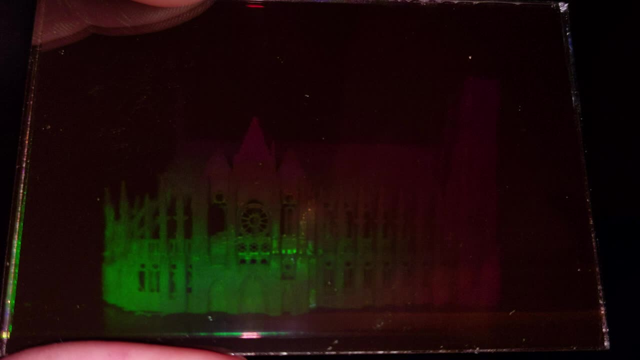 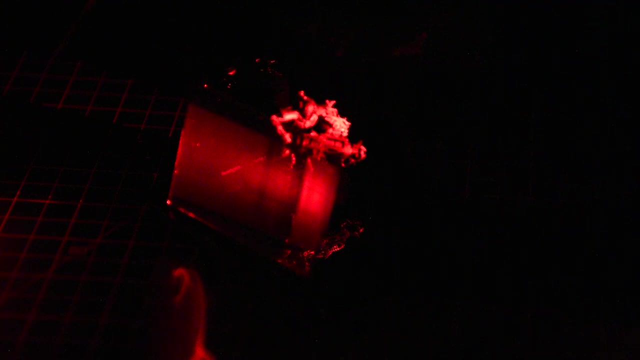 It simplifies everything so much, and is why I'm so happy they were willing to sponsor this video and send me some materials. Now, since this is a photograph, this will all need to be done in the dark Also, unlike a regular photo. 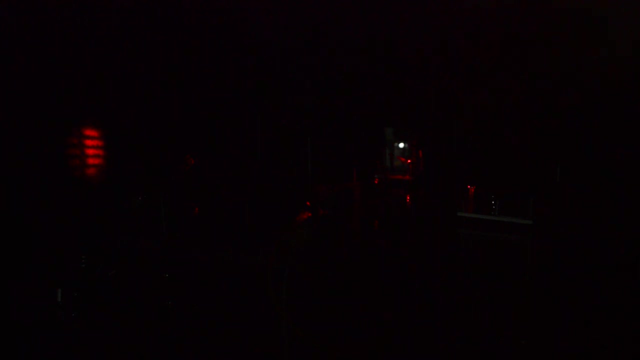 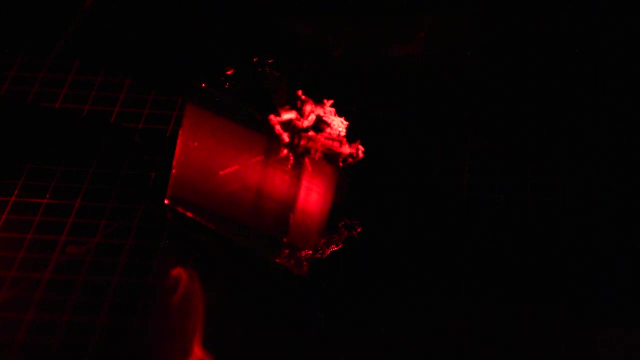 as we saw with the interferometer, holograms are quite sensitive to vibration, So you need to set this up on as large and heavy of a table as possible and turn off any sources of vibration in the room for best results. For me, this meant turning off all of my fans. 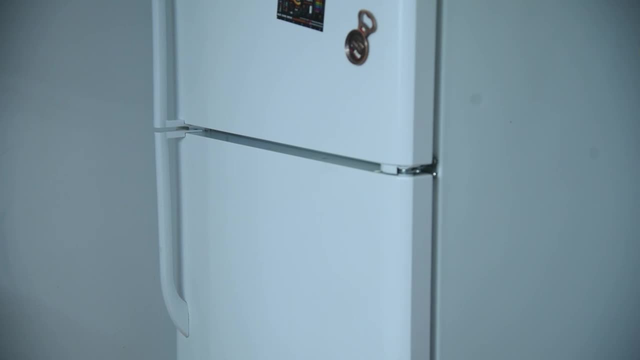 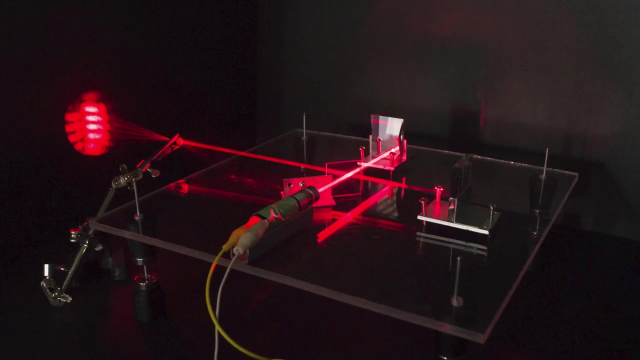 unplugging my fridge and unplugging or turning off any lights in the room, Just to be extra safe. I also did this late at night, so my neighbors aren't banging me around and there's less cars going by, But you don't need to do that. 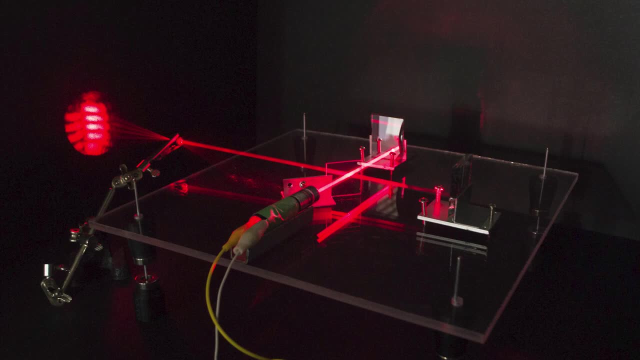 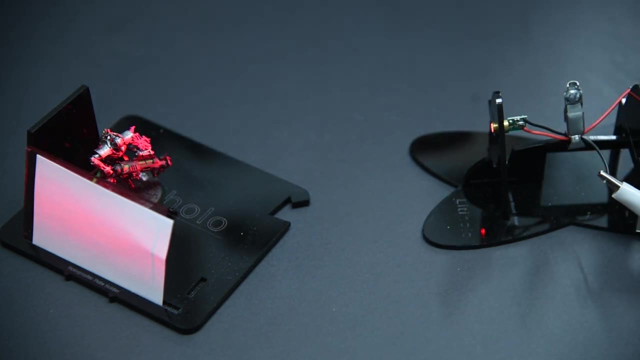 you don't need any special laser table or anything fancy, Just some basic precautions. First I'm going to turn on the laser and give it a few minutes to warm up and stabilize. Then I use a blank glass plate and a piece of white paper in the film slot. 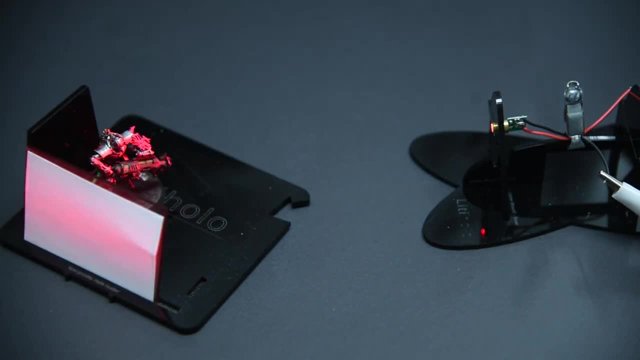 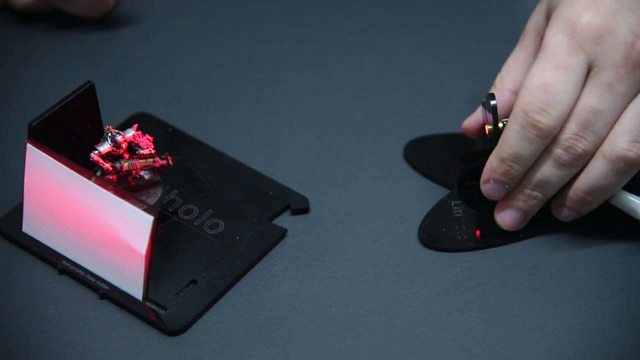 to line up the beam. You want the beam to completely cover both the plate and the object you're going to image, making sure the object doesn't get in the way of the plate and make a shadow. Obviously, this means your object should already be in place at this point. 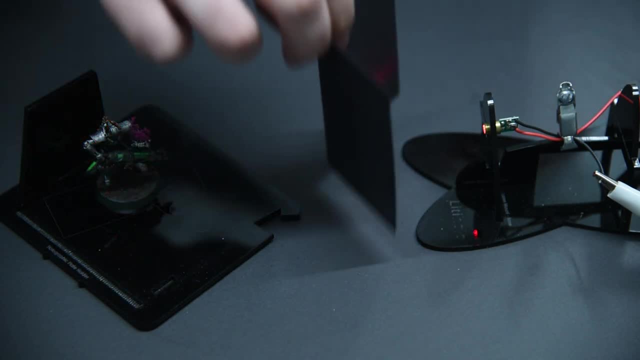 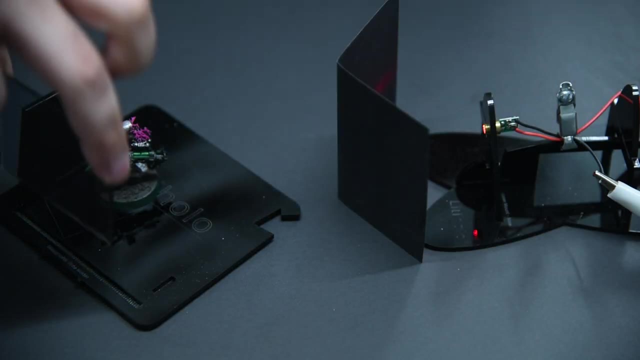 The glass plate is then removed and a black piece of cardstock is used to block the beam. Then, in the dark, I'll remove a film plate from its protective bag, place it into the film slot, and then it's time to wait. 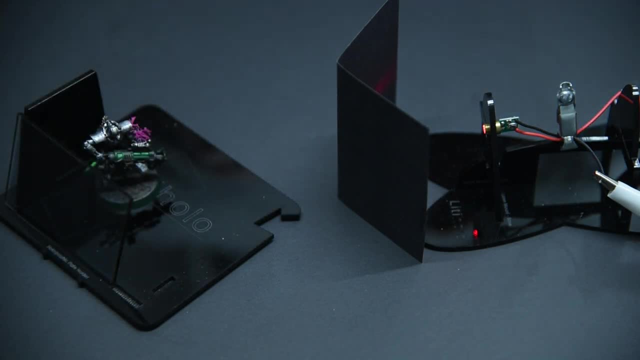 I'd highly recommend sitting comfortably for this bit, as you're going to need to sit perfectly still and make sure there's no noise in the room for a couple of minutes. This gives everything a chance to settle and all the vibrations to go away before the exposure. 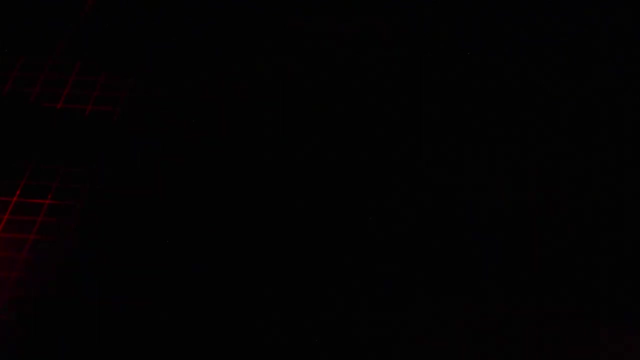 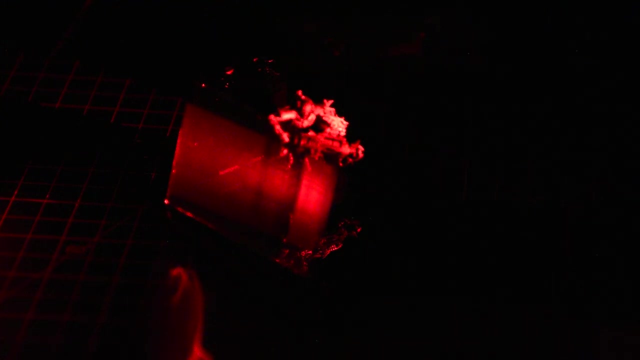 Then- being very careful not to shake everything- in one smooth motion, the black card is picked up and the beam is allowed to strike the setup. If you move slowly, you can place the card on your lap, so you're comfortable. Now again, hold perfectly still. 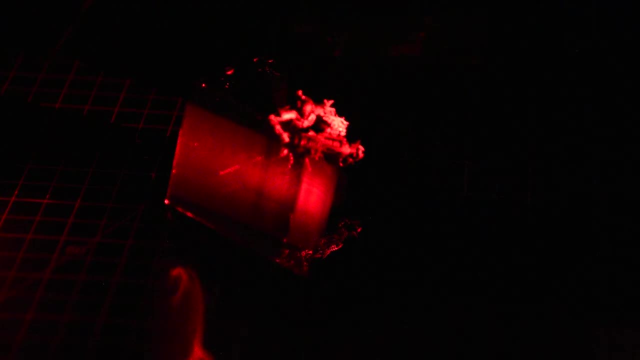 and try not to make any noise or breathe on the setup. The nice thing with this film is it's basically impossible to overexpose, so the longer you can sit still the better your image will be, but 3-5 minutes is usually enough to get a good image. 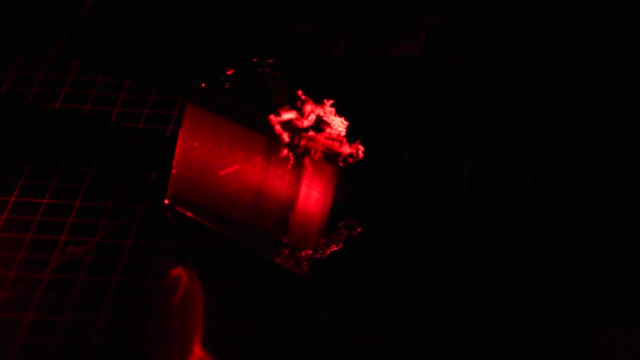 You can go up to 20 if you've got the patience of a monk, but I can't sit still that long After the exposure is done. place the card so it again blocks the beam. then remove your object from the stage and lift the card again. 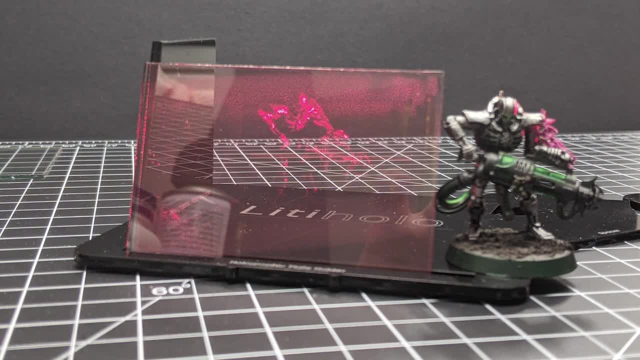 You don't need to be delicate about this bit. the exposure is already over. Now you can just view your newly created hologram. The best part of this film is there's no post-processing, so the hologram is viewable immediately, Sort of like an old Polaroid film. 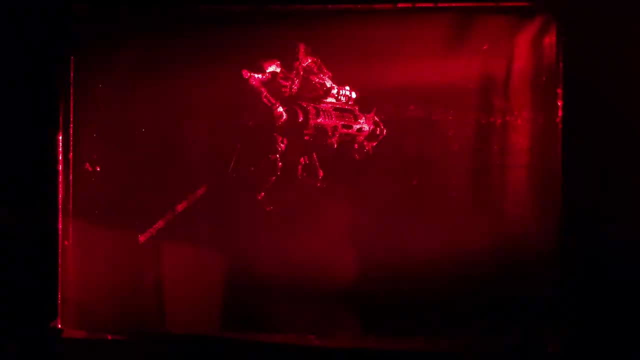 In my case, I now have a lovely view of a Necron from Warhammer 40k which I'd borrowed from a friend. Okay, so that's a transmission hologram and I made a few of them, but, like I said, 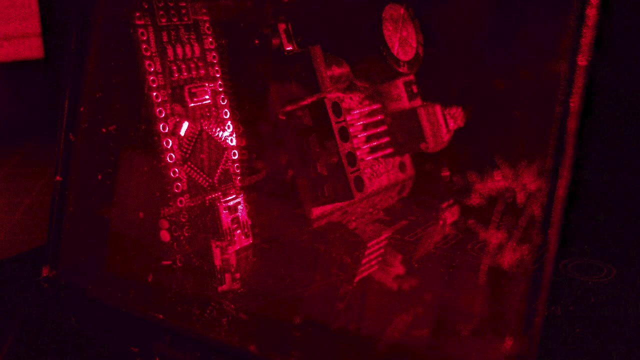 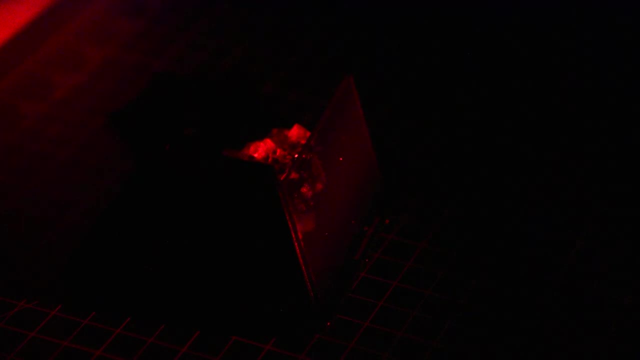 it requires laser light from behind to view, which isn't ideal for display purposes. So let's spin things around and make a reflection hologram. The setup is basically the same, but we spin the stage around, so the object is now behind the film. 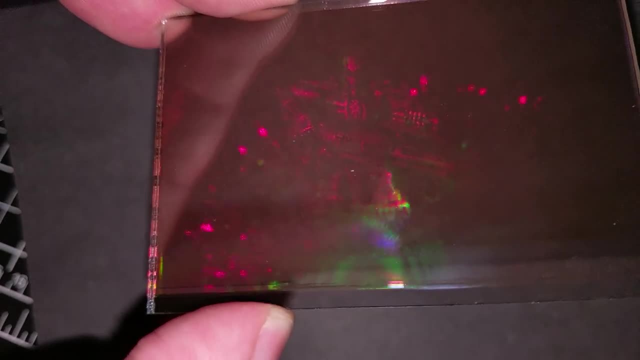 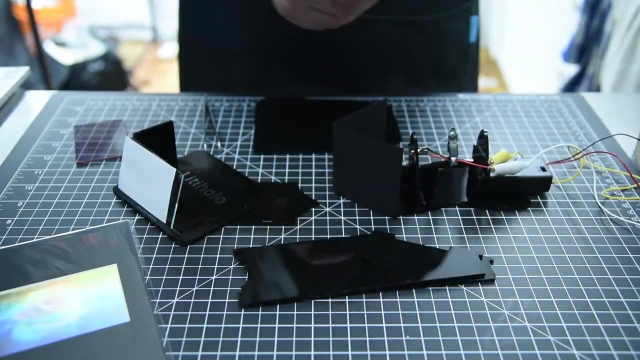 and the beam will hit the film first. I find these much easier to set up as well, and the angle of the object is nicer, since you're looking at it head-on rather than tilted to one side. Litty Hollow actually sent me their reflection kit. 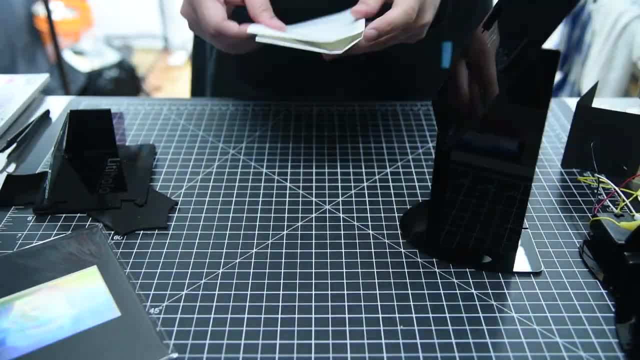 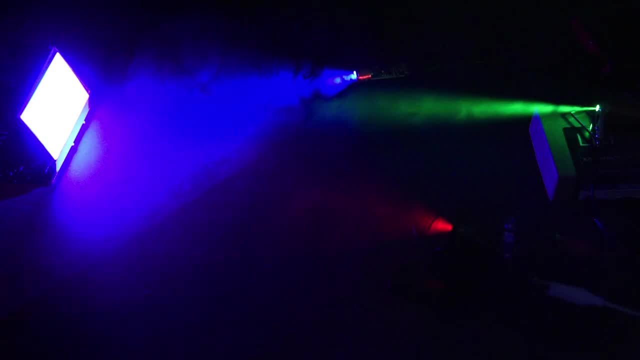 which comes with an extra stand to mount the laser on, but I found it easier to keep things the way they were and not bother with it, And this will be important later when we make rainbow holograms, as I'm not able to mount all the other lasers on the stand. 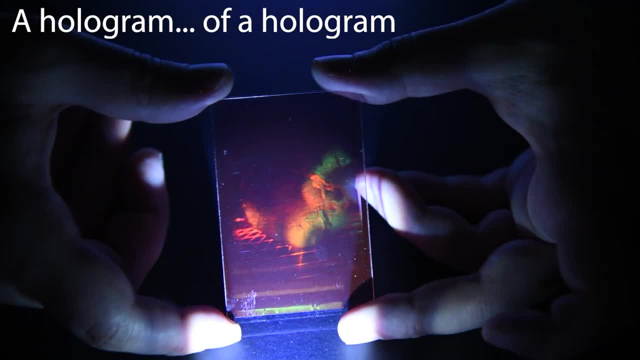 One note, though, is, if you use the setup this way, the final holograms need to be lit from a low angle because of how the plates are tipped, and that was how I made most of my holograms- A really easy fix to this. 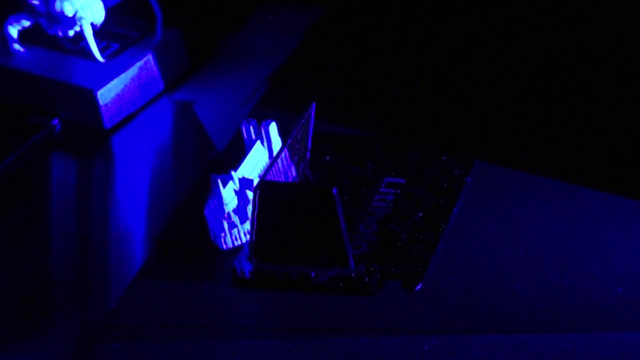 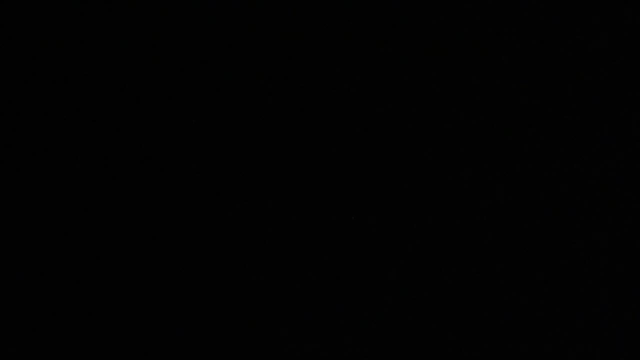 if you want to light them from above is to just spin the base around and raise the object up a bit, so it's still level with the base plate. The actual recording process is exactly the same as last time. First we kill the lights. 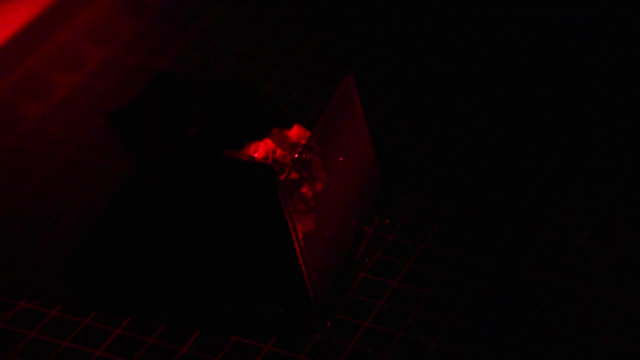 and any sources of noise or vibration, and then we block the beam In the dark, place a fresh film plate in the slot, wait for vibrations to come in, wait for vibrations to subside and then do the exposure just like before. 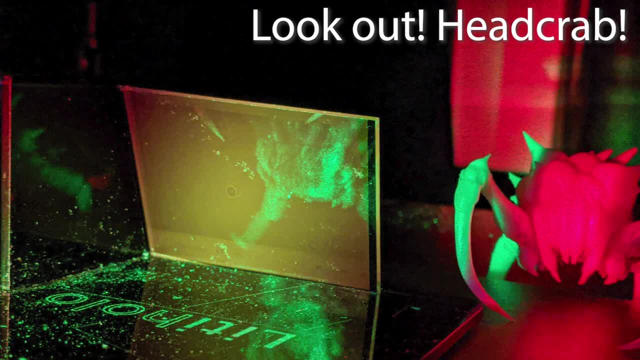 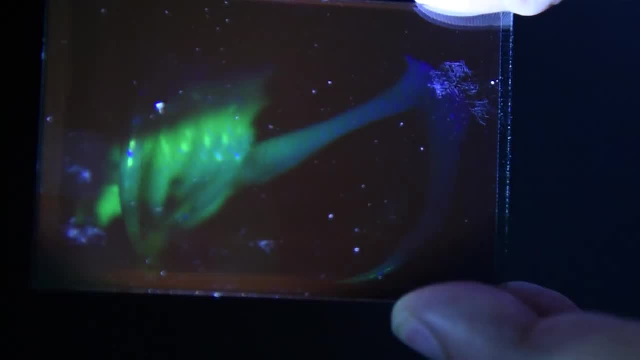 The result, though, is much different than the transmission holograms. Now, no laser light is required to view them, and a simple flashlight from the front allows the hologram to be seen clearly. Another quick note about lighting a hologram for display. 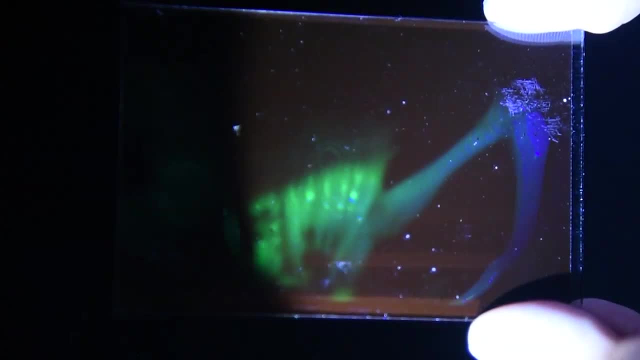 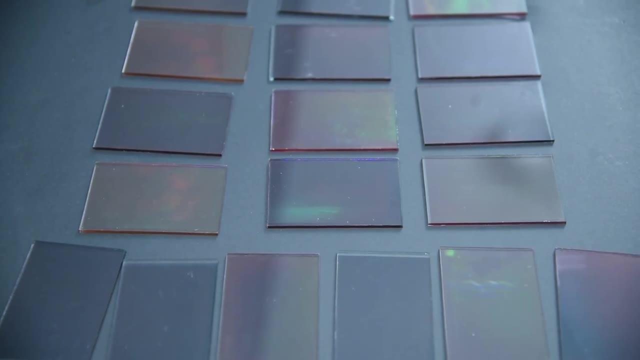 is that, for best results, you want a point source of light, something like a light bulb or a flashlight, rather than the long tubular lights I normally use for illuminating my work area. If you try and use the long lights, the hologram is often obscured. 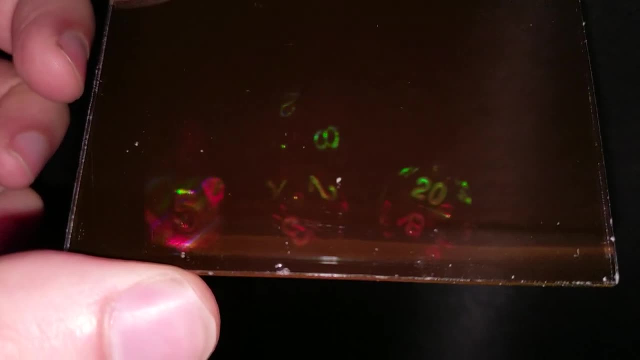 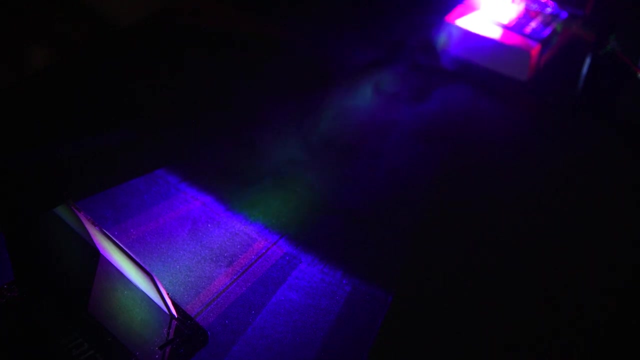 This is why the holograms don't look nice if I'm recording with my phone or a little LED flashlight, but is basically impossible to see under the normal work lights. Okay, before we talk about using different colored lasers or making the rainbow holograms, 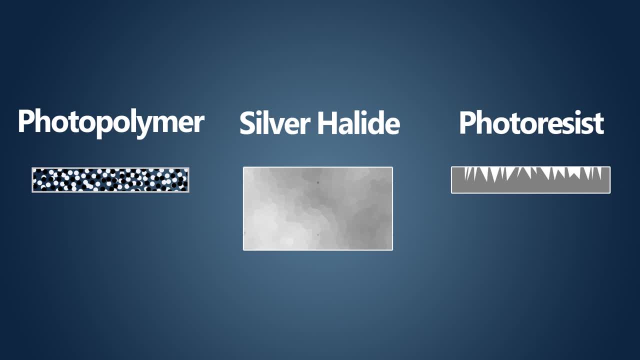 I want to talk about the film I'm using. You see, there's actually many different recording media options to choose from. I just happen to like this film because it's so much easier to use. Traditionally, though, making holograms normally takes a lot more work. 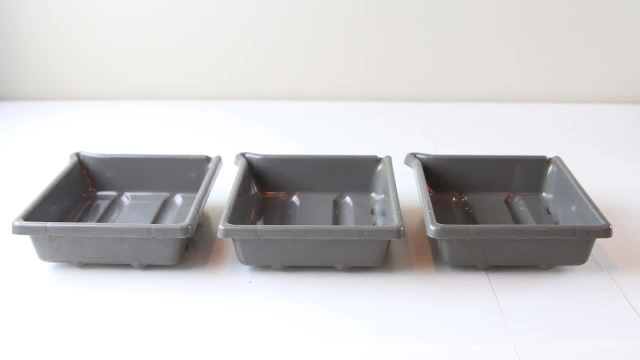 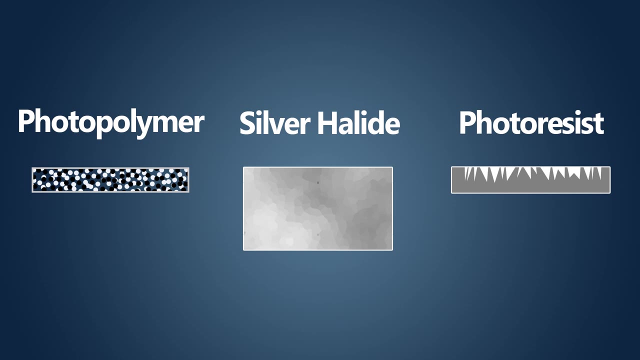 That's because most of the other options need to be treated like old school photographs, where, after the exposure, they need to be developed and bleached in a dark room to reveal the hologram. However, each recording media also comes with various pros and cons. 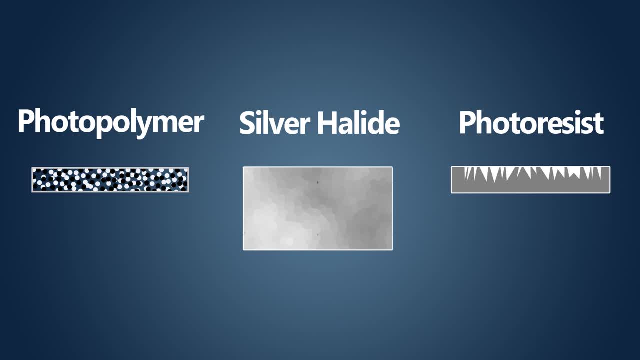 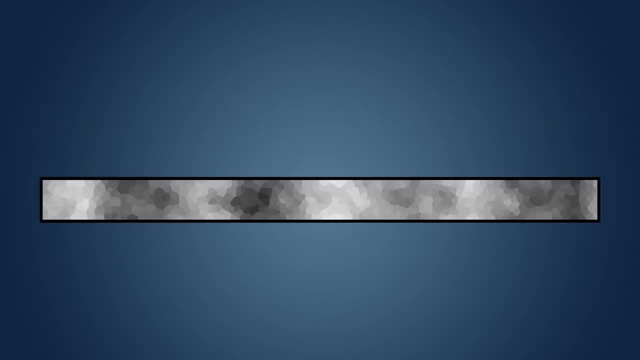 and changes what the end hologram will look like and what it can be used for. The film I'm using is a photopolymer, so areas where the interference pattern make a spot brighter will react more than areas where it's darker. In this case, the bright areas polymerize. 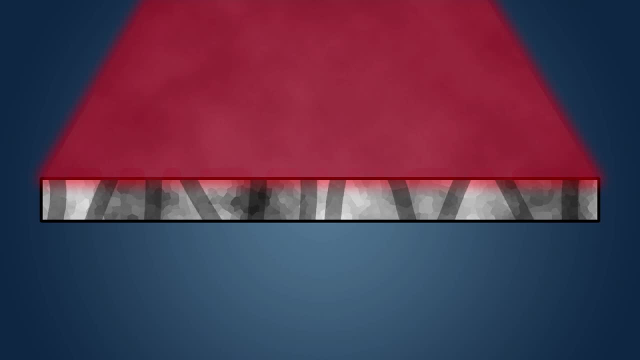 which means that they chemically link together and get denser than the dark areas. As the exposure proceeds, the chemicals in the film get depleted, so once the hologram is made there's no more reactants left, so the dark areas can't polymerize and ruin the pattern. 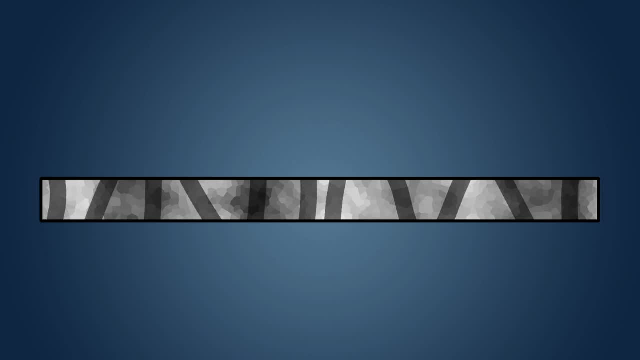 This is why there's no developer needed with these materials. There's no need to wash away unreacted areas to make the hologram be visible. What makes this particular film great is that the chemical reaction isn't that picky about the color of light that's used. 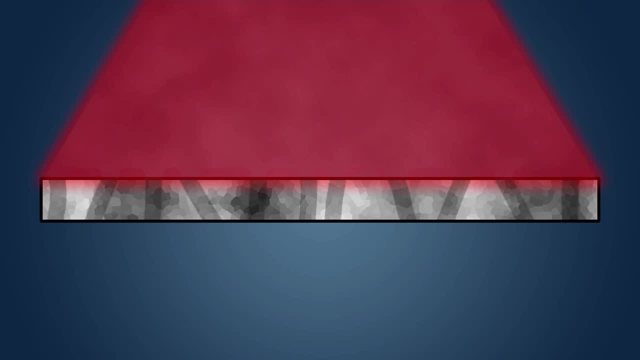 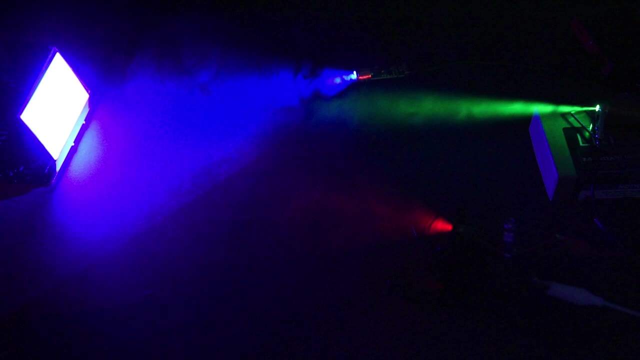 It prefers red and reacts most strongly with that, but can also work with green or blue, just more slowly. However, the color used does change the exact nature of the reaction and make the hologram that gets recorded look like the same color that was used to make it. 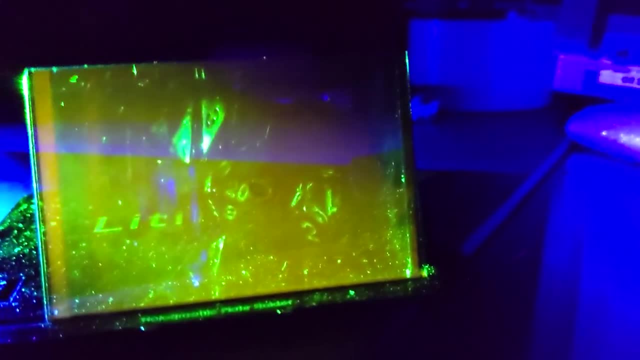 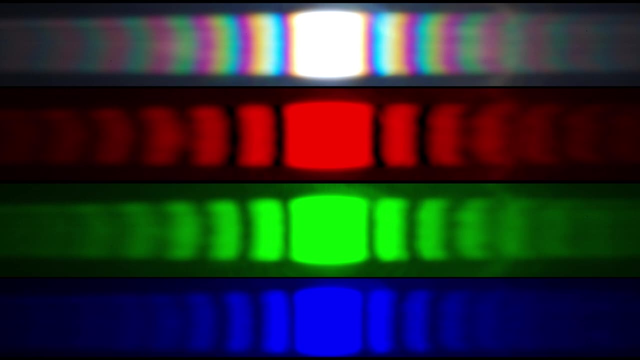 So red lasers make red holograms, green make green and blue make blue, And if you use all three at once it'll look whitish. if you balance things properly, This is because the wavelength of each color is longer or shorter, and the interference pattern. 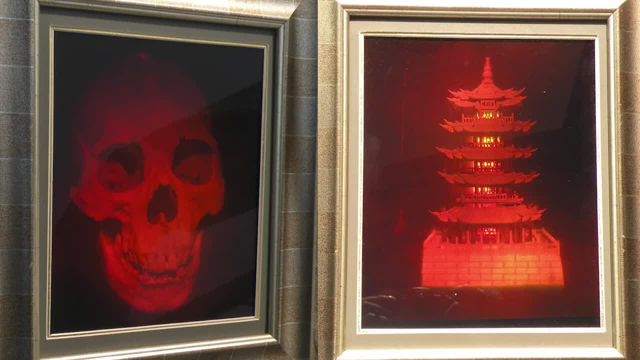 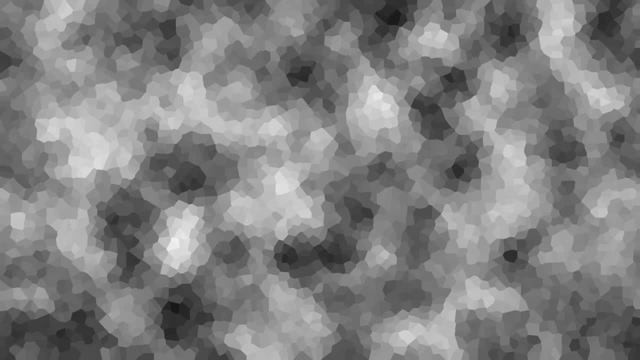 will be larger or smaller accordingly. A more classic material is silver halide suspended in gelatin. These are exactly what a regular photograph uses. It's tiny grains of usually silver chloride that are only a few nanometers wide, suspended in gelatin and then spread onto a glass plate. 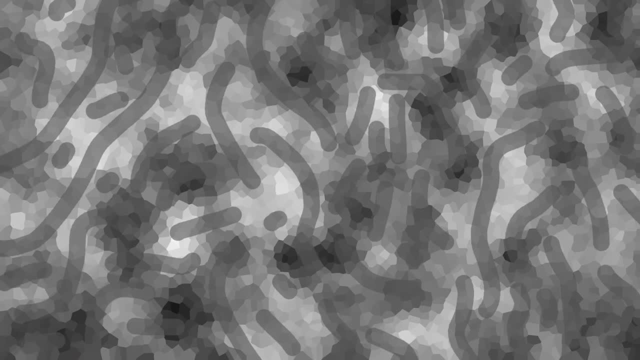 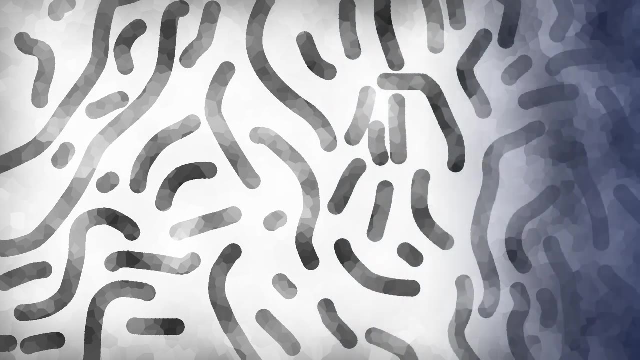 When light hits the mixture, known as an emulsion, the silver salt actually sheds the chlorine atoms and turns into pure silver metal. The development process will wash away any unreacted salts and permanently fix the silver metal in place. The difference between this. 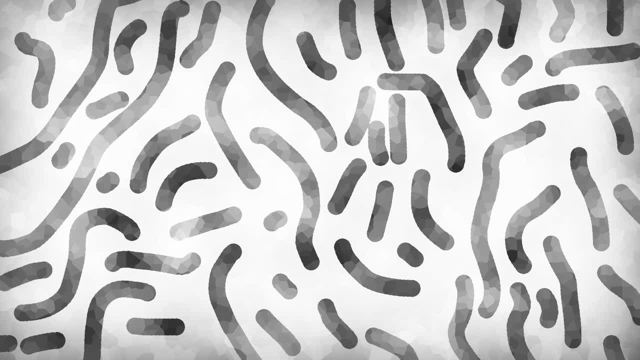 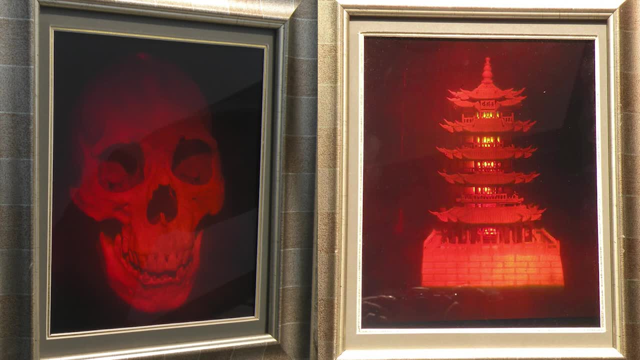 and a regular photograph, though, is the size of those silver grains is much, much smaller, so the interference pattern can be recorded in the pattern of the silver metal. One benefit of this, though, is often the end result is a much brighter hologram. 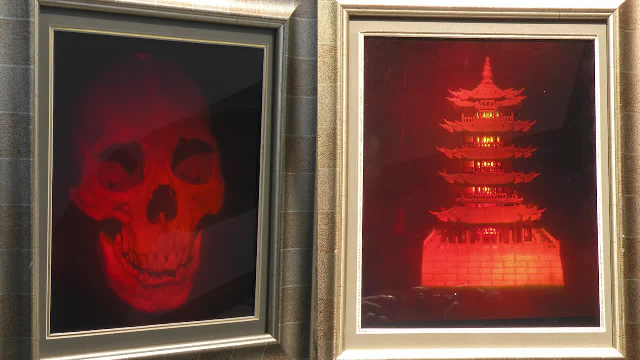 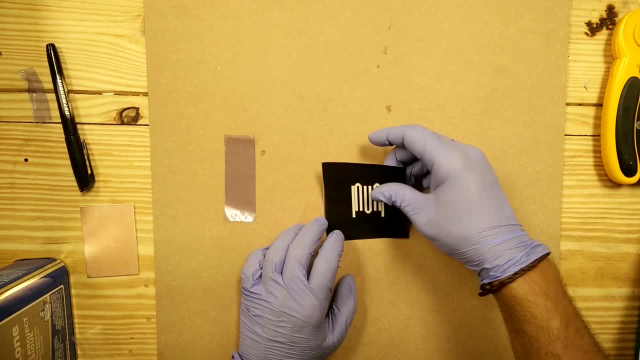 and only the hologram itself is visible, with no colored backdrop. And finally, there's photoresist. This is very similar to the photopolymer in that it's a chemical that's spread on plates. If you've ever made a circuit board from scratch, 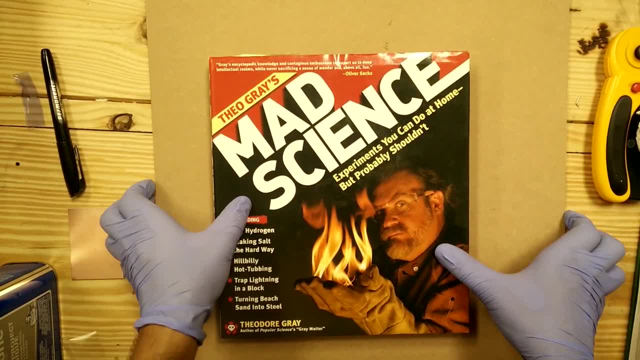 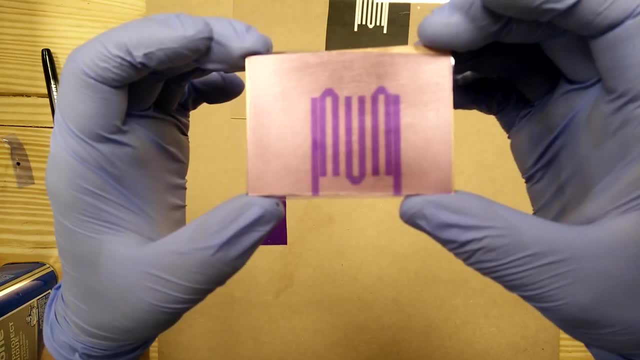 you may have used photoresist before. The idea is you shine a blue or UV light on it, and areas that are struck by the light chemically react and polymerize, whereas dark areas don't just like the photopolymer, But unlike the photopolymer. 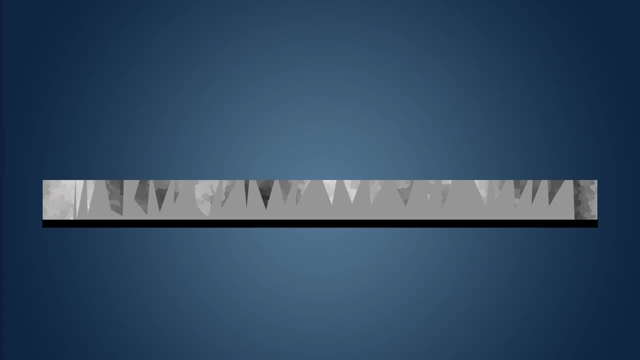 the final step uses a solvent to wash away any unreacted photoresist. This method is special because, unlike the silver halides or photopolymer, instead of the pattern being recorded as darker or denser areas, the hologram gets recorded as a physical pattern of bumps on the plate. 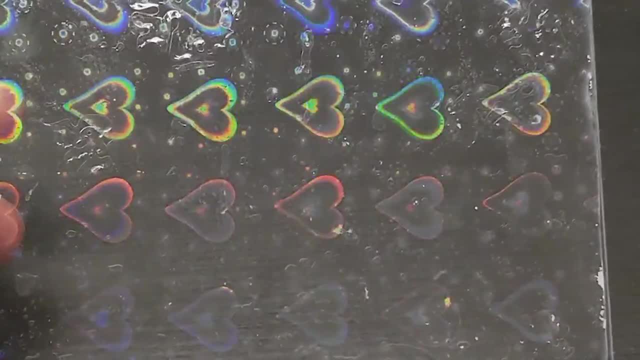 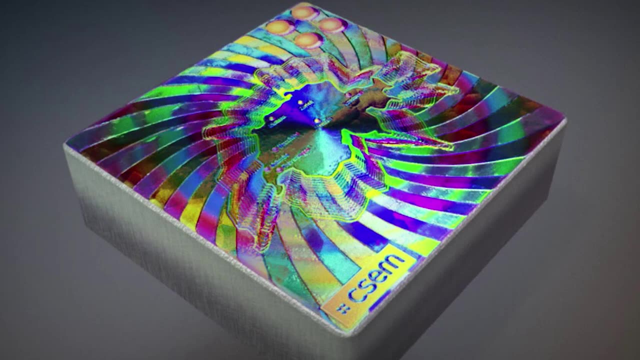 This is useful because you can make a physical cast of those bumps and then transfer that pattern to other things very easily. If your cast is made of metal, you can heat that metal up and press it into plastic to instantly transfer the hologram pattern to that plate. 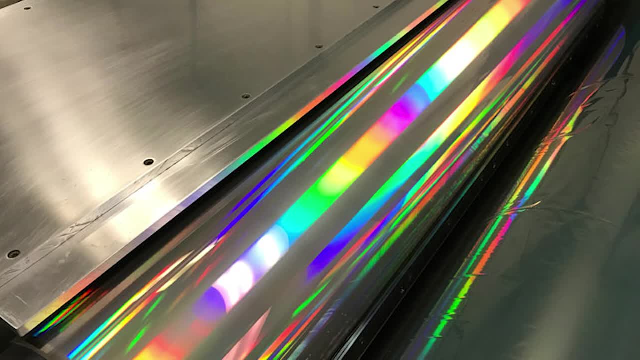 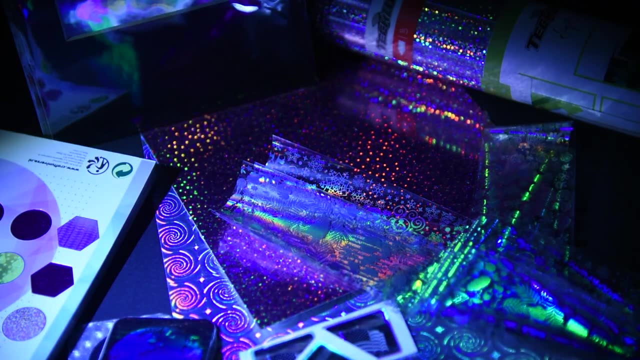 This allows rapid mass production of holograms very easily. If you've ever seen these products with a rainbowy sheen or these bright rainbow patterns, that's actually how they're made. A metal hologram mold is created and then hot stamped onto plastic. 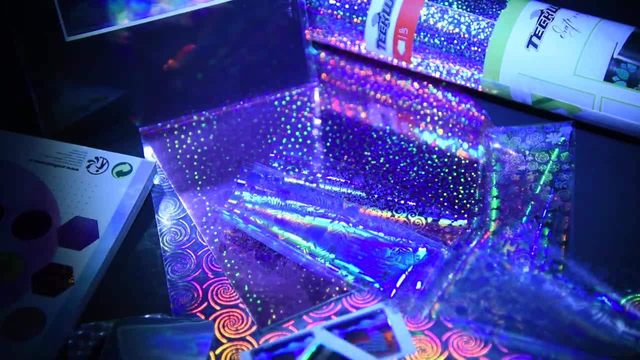 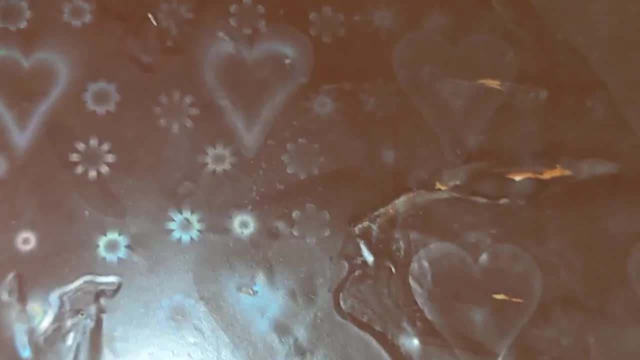 to make it holographic. These types of holograms are known as embossed holograms. Ben over at Applied Science actually showed that the same thing can be done with chocolate and made chocolate holograms by using commercially made embossed holograms and transferring their pattern. 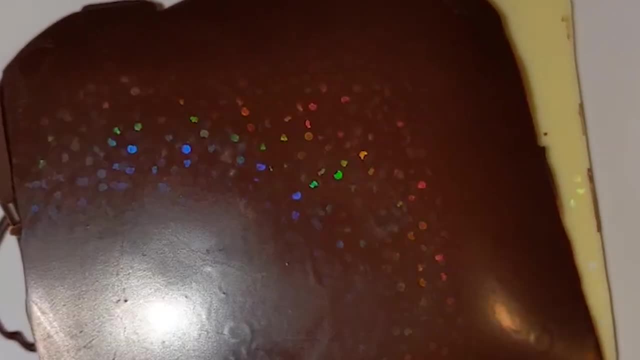 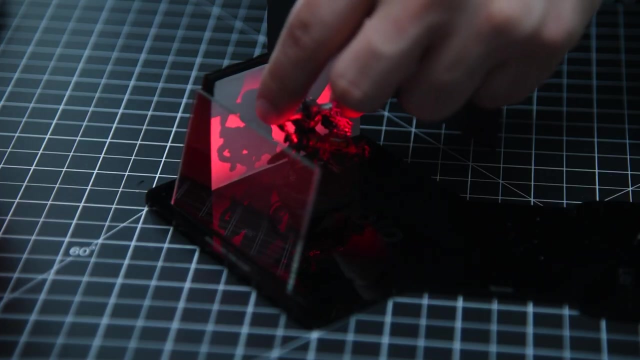 to some chocolate. I've been working on the same thing for quite some time and will be making a video building on his method and showing some improvements I've been tinkering with soon, But I wanted to make this video first so you understand how holograms work. 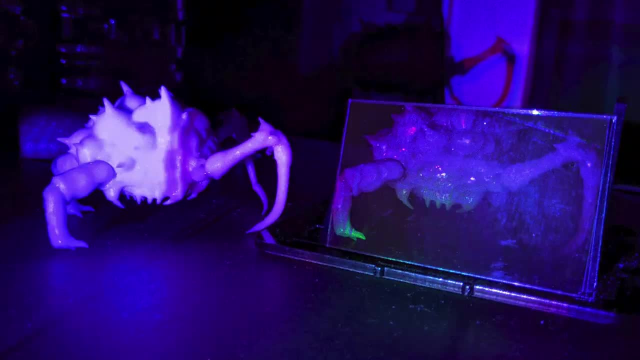 so I can focus on the mechanics of the embossing method in that video. Okay, so now that we know how the film works, let's make some rainbow holograms. My first thought was to get three different lasers: a red, green and blue. 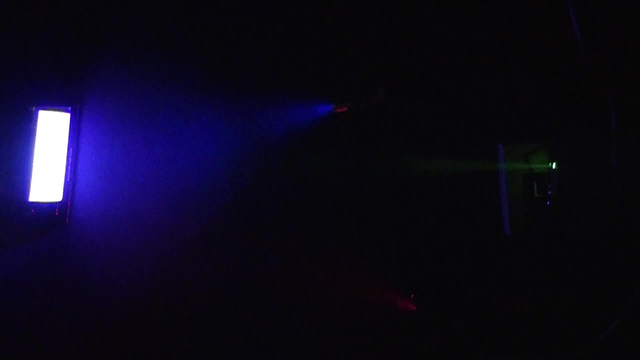 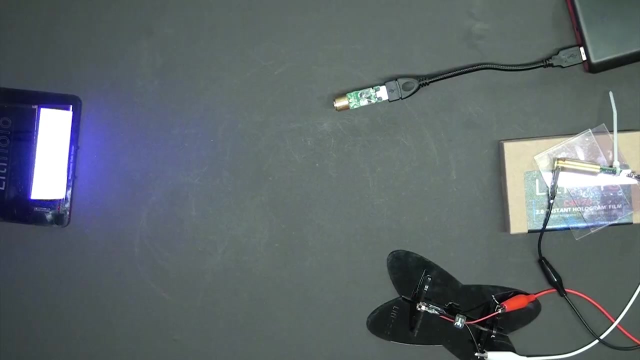 and just shine them from far away onto the film so they overlap and seem like they're all coming from the same direction. The red laser is the one from Liddy Hollow, but the green and blue ones came from Amazon. The blue was by far the trickiest to find. 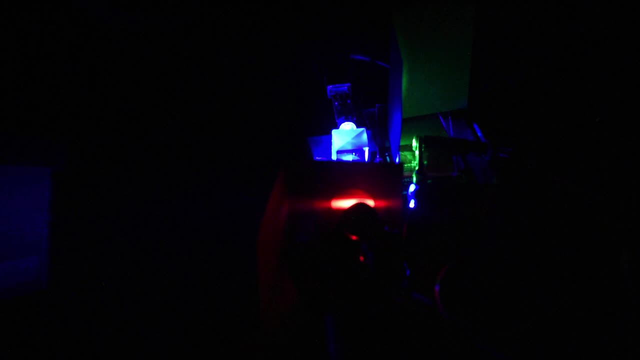 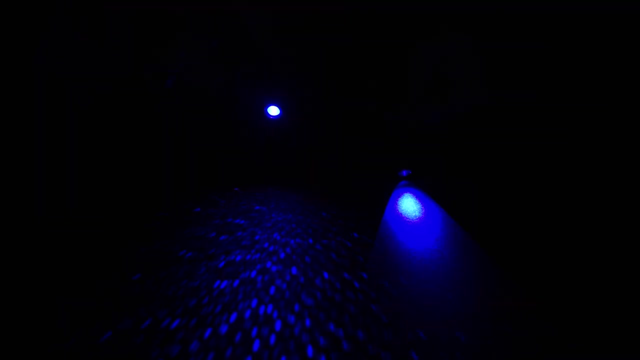 since most blue lasers are actually violet and entirely useless for this. What I ended up finding that worked was this blue laser star decoration thing. It projects a pattern of dots on the ceiling when you plug it in but, importantly, it contains a proper blue laser. 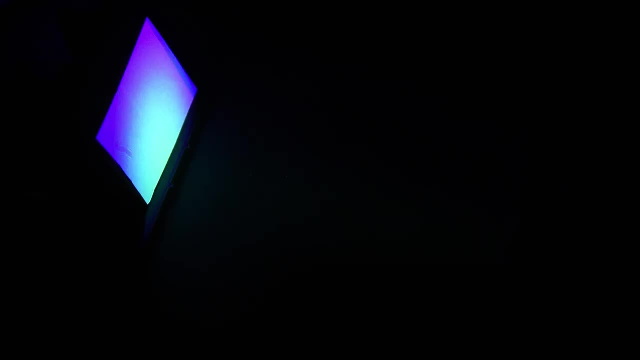 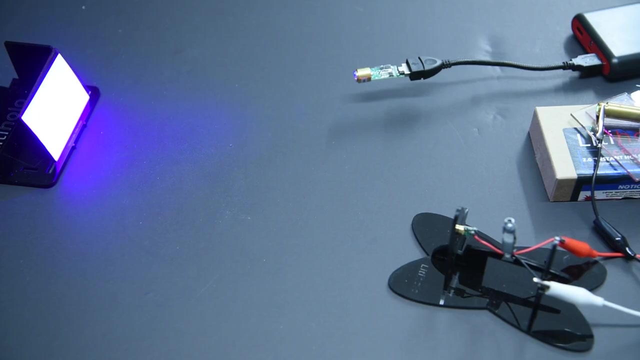 So this was gutted to reveal the perfect blue laser. You can see that when all three lasers are aimed at a white piece of paper, the colors all mix and appear whitish themselves. Unfortunately, my original plan of just aiming them all at the film. 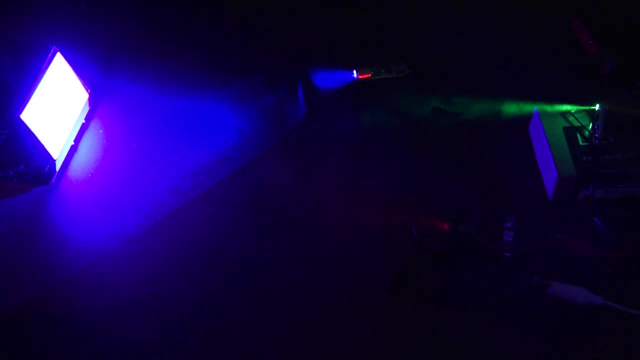 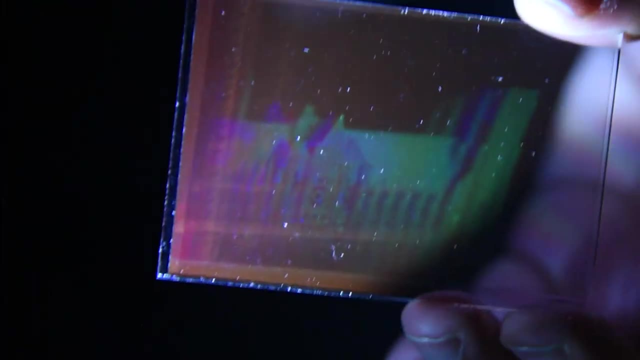 didn't quite work. You can see that the two lasers on either side are tilted at a slight angle, and this slight angle gets recorded in the hologram. So the final hologram. it looks as if there's three separate objects, one in each color. 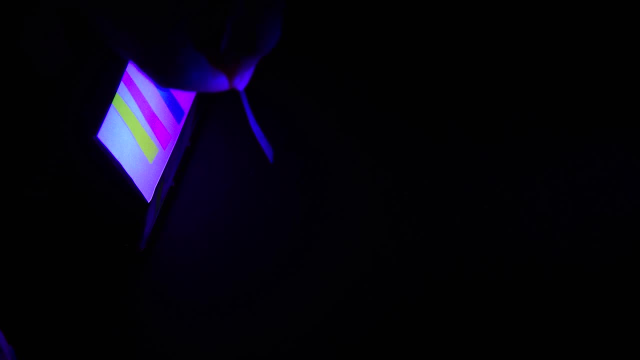 that don't quite overlap. If I put something in the path of the beam, you can see this as three very distinct, separate shadows. So what I need to do is make it so that all the lasers come out in a straight line and go directly to the film. 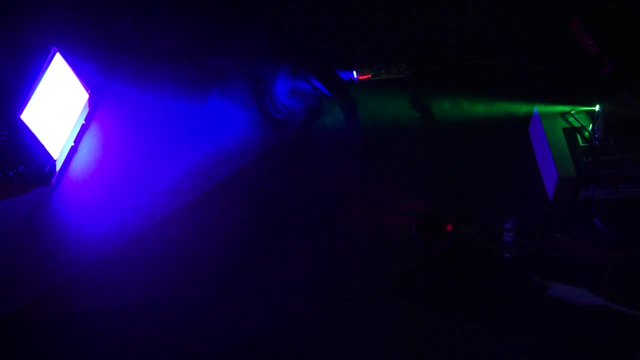 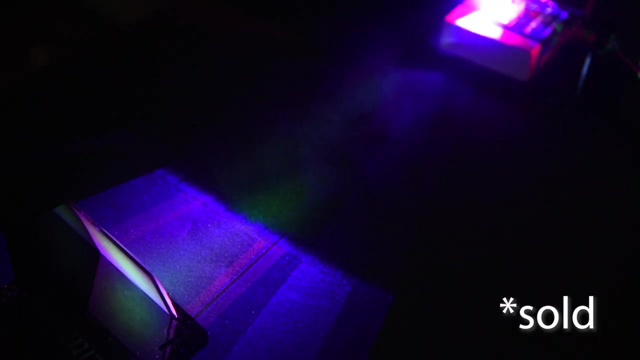 But I can't just aim the lasers in the same direction, or only one of them would actually hit it, So I need to combine all three beams into one that can just be aimed at the film. Liddy Hollow actually sells a kit to do this. 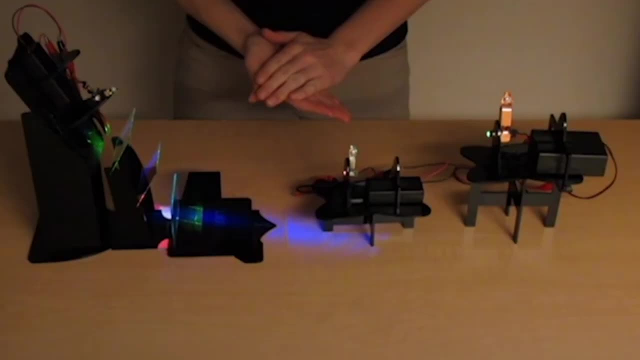 and their kit uses dichroic mirrors that each allow some colors to go through while reflecting others. But getting those special mirrors can be annoying and expensive, so I wanted a cheaper and easier solution. I ended up picking up some of these beam splitter cubes. 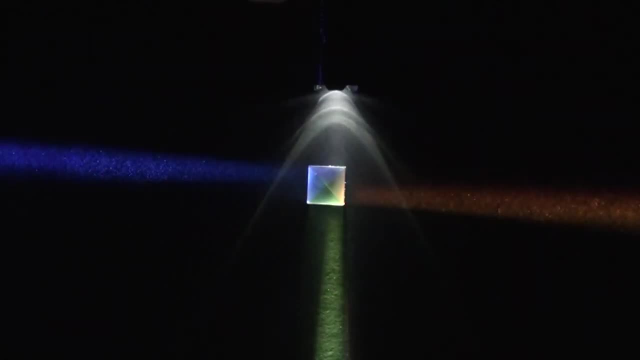 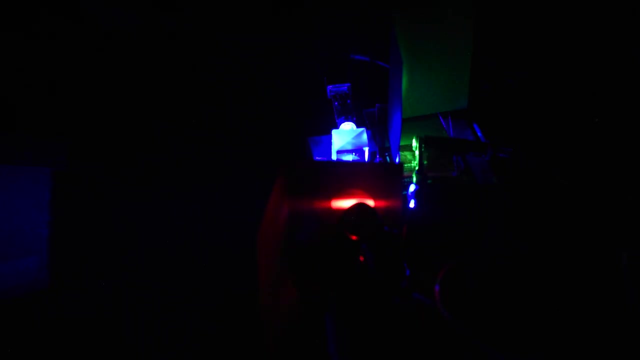 which can be purchased on Amazon for a few dollars. These are neat because normally you can shine a white light through them and get three colors coming out the other sides. So I simply did this in reverse: I shined three colors in the sides. 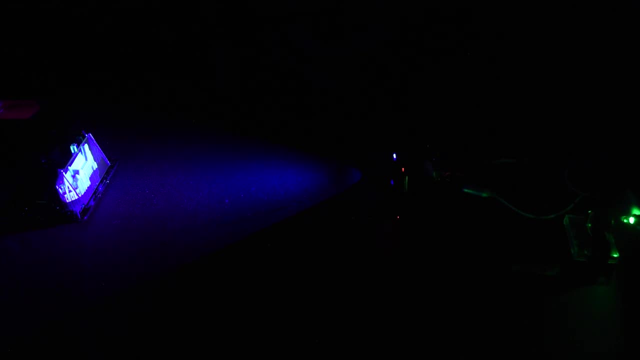 and get white light out the front, Rather than any kind of delicate setup. I just kind of piled things up that I had on hand and took some time to line up all the lasers and within a couple of minutes I had a nice white beam. 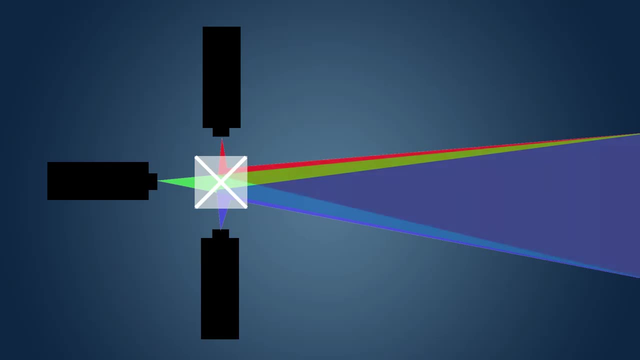 I could use for the exposures, Since the film is less sensitive to different colors. to get the best results, you either need to adjust the laser power of each beam so that they're all even, or change how long you leave them to leave each exposure open for. 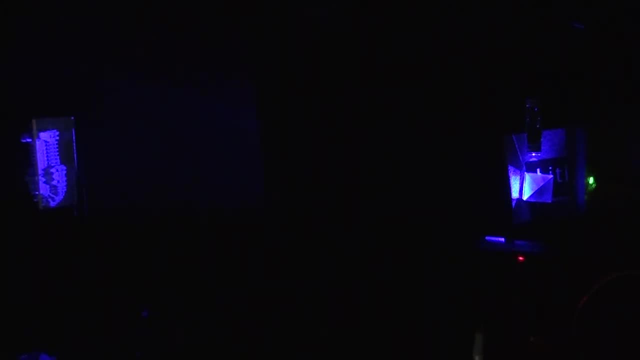 I can't change the power of these lasers, so instead I would just unblock each color successively. First I'd let the blue laser work for a couple of minutes, then I'd add red, and then, finally, I'd add green. 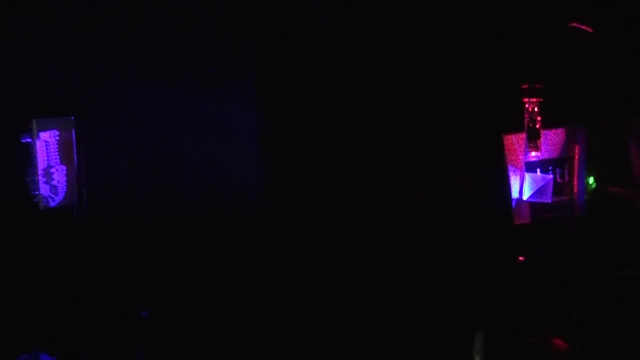 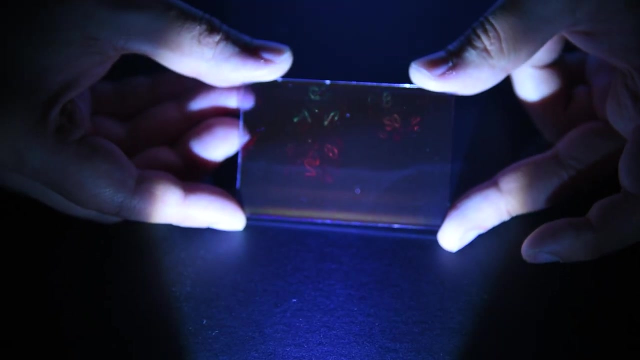 since my green laser is actually more powerful than the other two. I took a bit of practice and experimenting to get the timing right. but when everything is perfect you get beautiful rainbow holograms. After I'd made a few of these and I'd gotten my timing down. 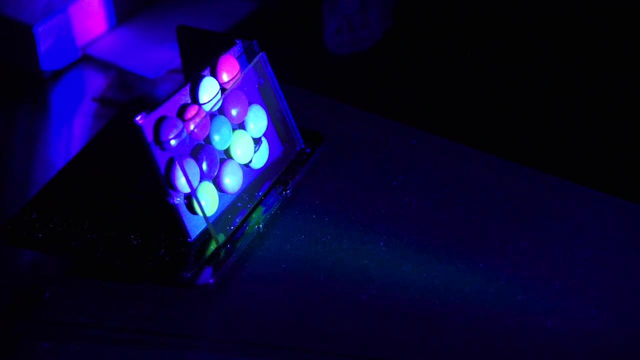 I wanted to see if using white light gives you any color information about the object that you're capturing. So I picked up a pack of Smarties which are basically like Canadian M&M's and glued some to a piece of cardstock so they all sit flat. 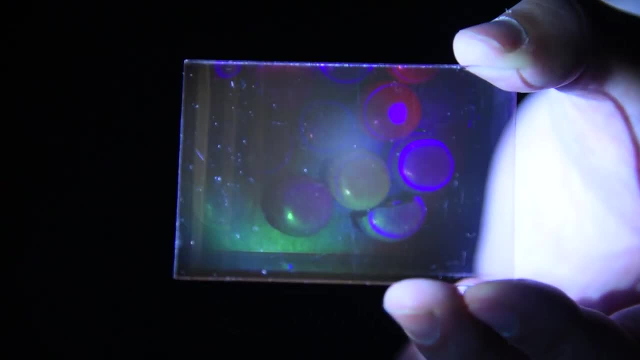 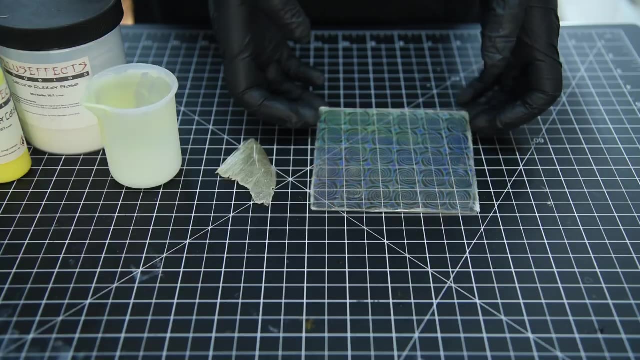 relative to the film plate. After the exposure, you can see that some of them really do look their proper color, which I think is amazing. But for now, that's where I'm going to leave it. Like I said, we're going to be coming back. 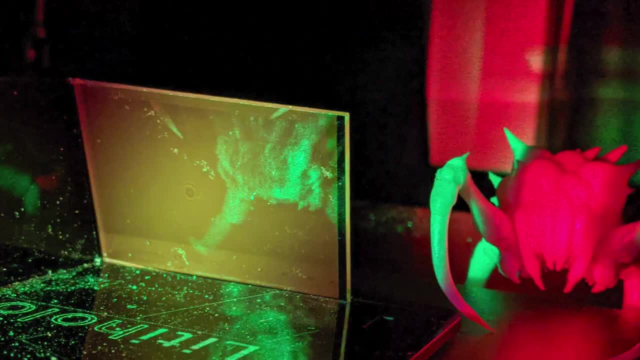 to holograms in a future video, because these are just too cool not to want to play with more, and I want to see if I can transfer some of these homemade holograms to chocolate and use them as my go-to cake decorations. So be sure to subscribe. 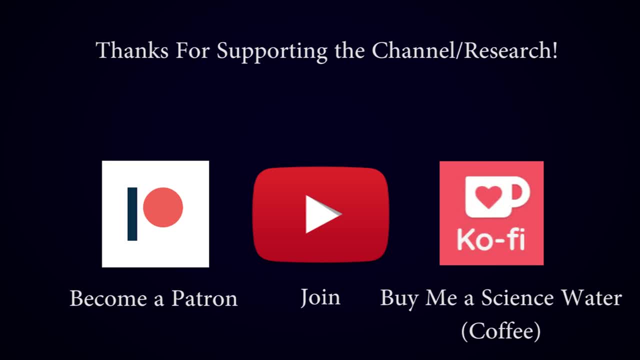 to see when that video is released. As always, I need to say a special thank you to my amazing patrons, channel members and supporters on Ko-fi that make these videos possible. Your support is the main thing that lets me make these videos. 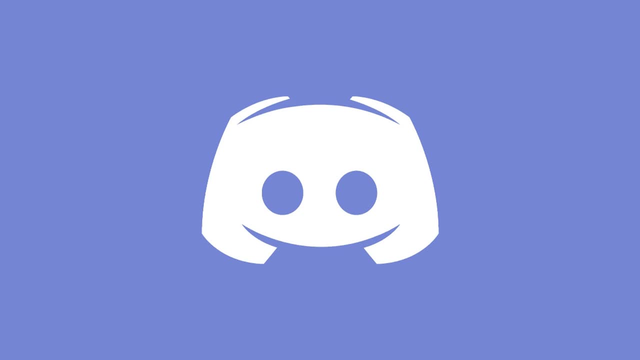 and I am so grateful. Patrons and members also get access to the Discord, so if that's something you're interested in or just want to help keep the flow of science videos coming, there's some links below If you enjoyed this video. 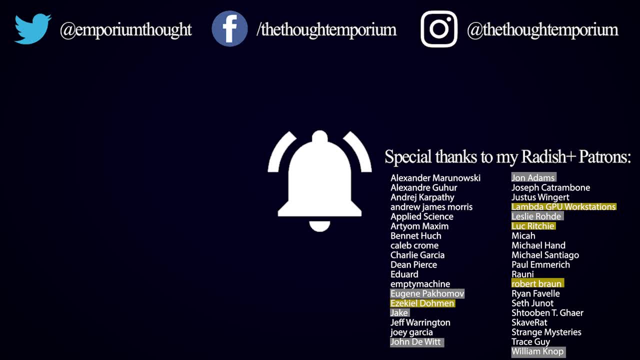 you know the drill: Hit that like button, subscribe and ring the bell to see when I post new videos And to see these projects long before they make it into videos, head over to my other social media pages, like Instagram. I've been posting snapshots. 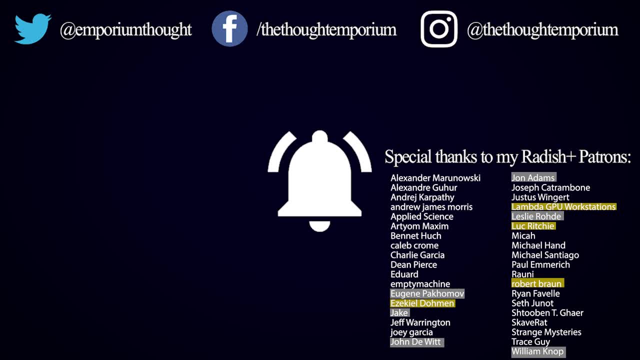 of this project for months on Instagram and Twitter, so people that follow me there know what I'm working on. That's all for now and I'll see you next time.